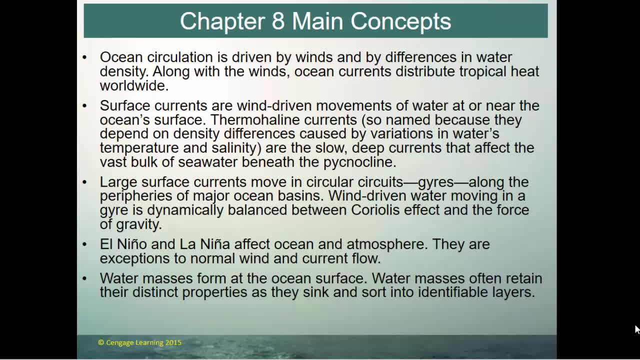 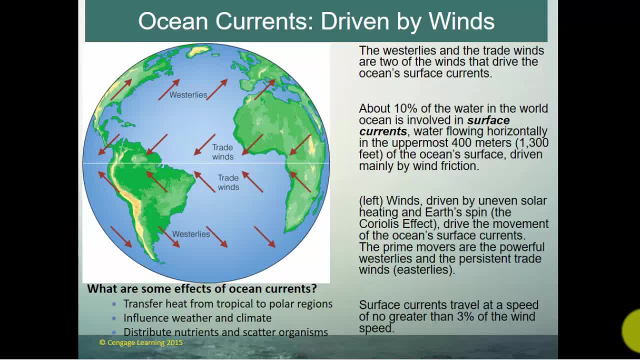 the ocean surface and how they retain their distinct properties as they sink and sort into identifiable layers. So, first and foremost, ocean currents are driven by winds. The westerlies and the trade winds are two of the winds that drive the ocean's surface currents, And you can see the 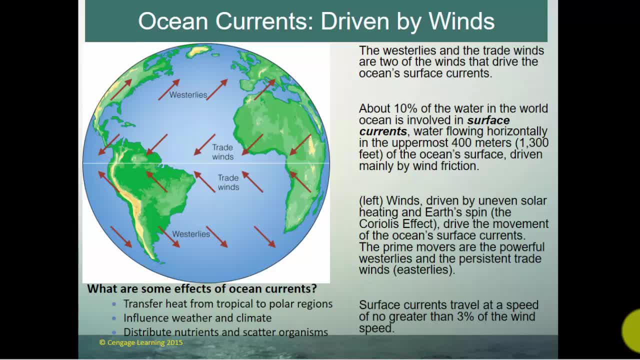 westerlies going to blow from west to east at the surface and the trade winds from east to west, And what that allows to happen is that you start to get a clockwise flow in the northern hemisphere and then a counterclockwise flow in the southern hemisphere. What that ends up actually looking like. 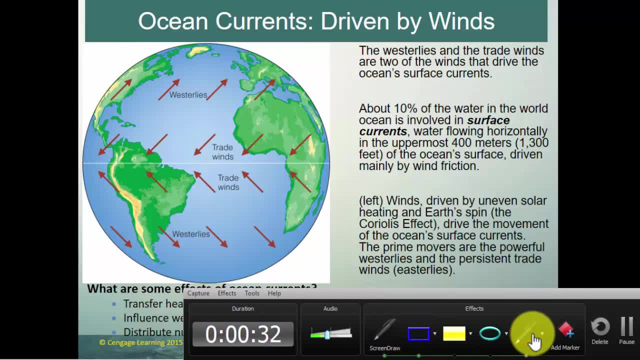 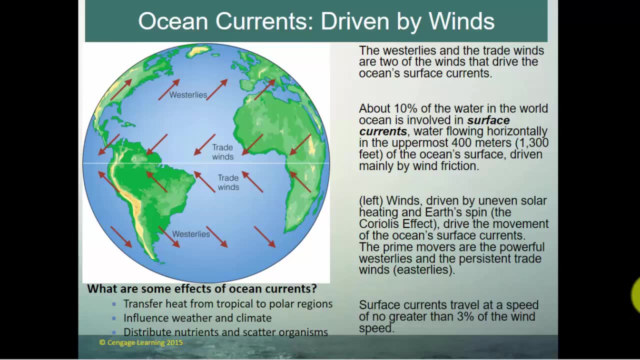 are these large, what are known as gyres, which are actually going to be the currents of the ocean, turning in a clockwise flow in the northern hemisphere and then a counterclockwise flow here in the southern hemisphere, And each of the main ocean basins has one of these large gyres. 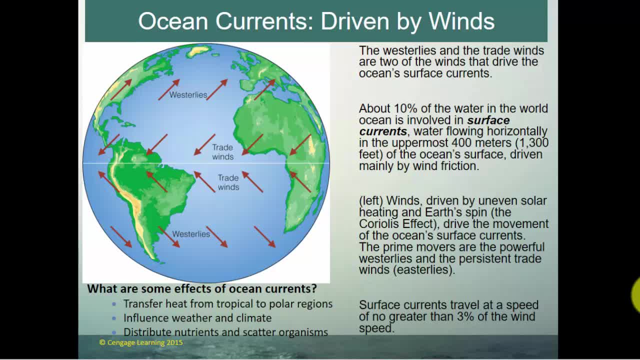 one of these circular flows. So about 10% of the water in the world ocean is involved in surface currents. Only that 10% water flowing horizontally in the uppermost 400 meters of the ocean, driven mainly by wind friction. So winds driven by uneven solar heating. Again, remember at the equator. 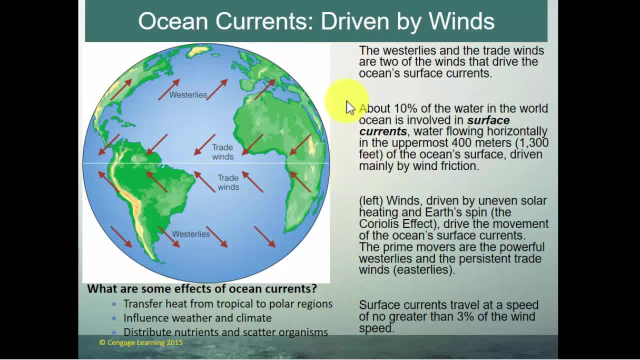 we heat up, At the poles we cool off. So air rises At the equator, moves north and sinks to the poles and moves back south. So winds are driven by uneven solar heating of the earth's surface. They spin due to the Coriolis effect and drive the movement. 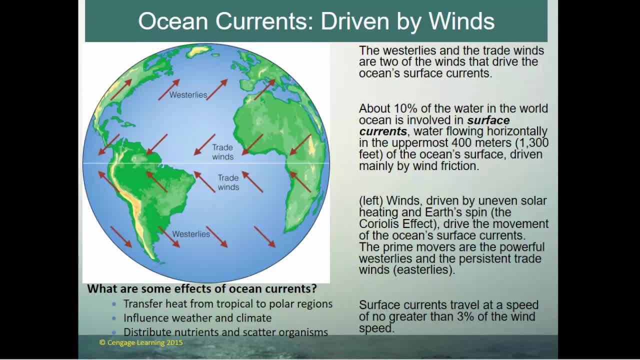 of the ocean's surface currents, The prime movers are the powerful westerlies and the persistent easterlies, those northeast and southeast trade winds. Surface currents travel at a speed no greater than about 3% of the wind speed. So if you have winds moving at 100 miles per hour over the 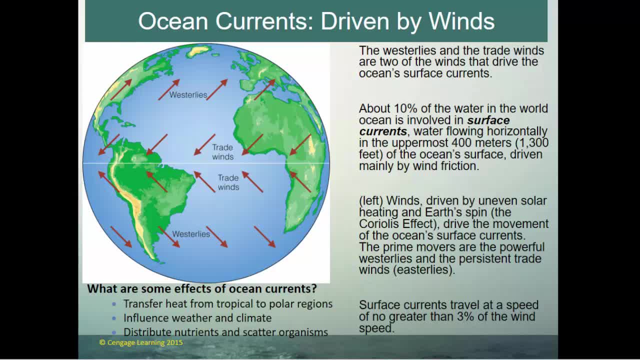 ocean surface currents only move there at about three miles per hour. So the wind really has to be lots and lots of wind to create these surface currents, lots of persistent wind. So what are the effects of those ocean currents? They transfer heat from the tropics to the polar regions. 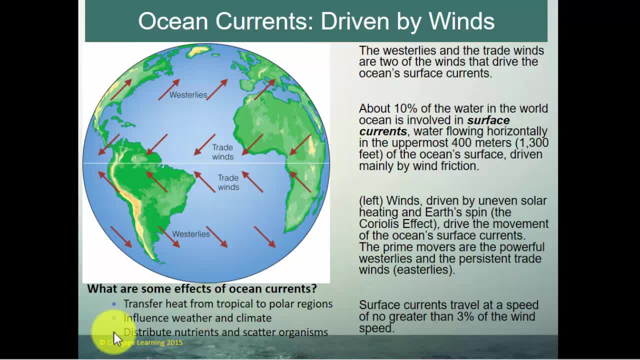 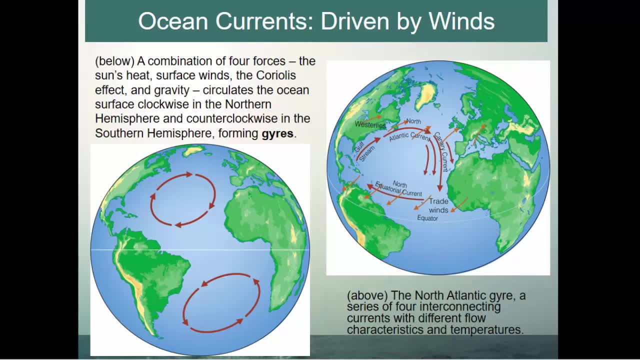 they influence weather and climate, and they also distribute nutrients and scatter organisms around the globe. So a combination of four forces- the sun's heat, surface winds, coriolis and gravity- circulates the ocean surfaces clockwise in the northern hemisphere and counterclockwise in the 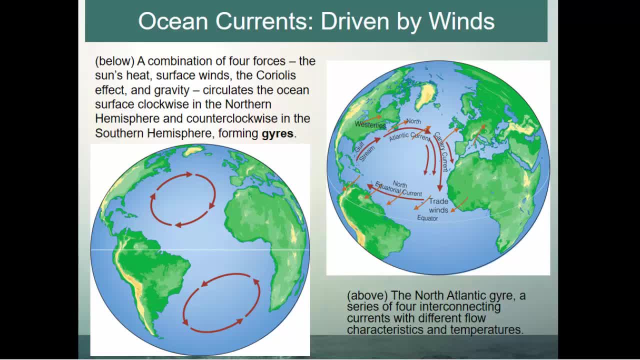 southern hemisphere, forming the gyres that we just talked about. So in this illustration. well, those are the two gyres that I showed you in the last slide In this illustration, the North Atlantic gyre, it's a series of four interconnecting currents with different flow characteristics and 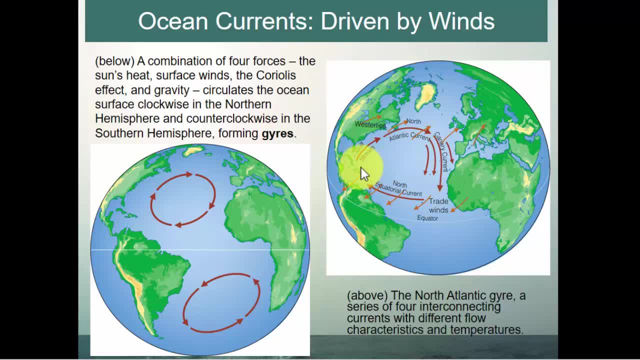 temperatures. You have the North Equatorial Current, you have the Gulf Stream, the North Atlantic Current and the Canary Current, And these currents are driven by the North Atlantic Current, driven by the Northeast Trade Winds and the Westerlies, and they result in this one large 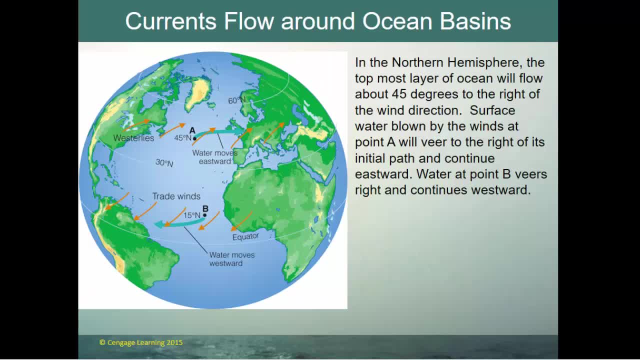 gyre in the North Atlantic. So in the northern hemisphere the topmost layer of the ocean will flow at about 45 degrees to the right of the wind direction. So it's the same in the southern hemisphere, but it's to the left of the wind direction. So let's just talk about the northern. 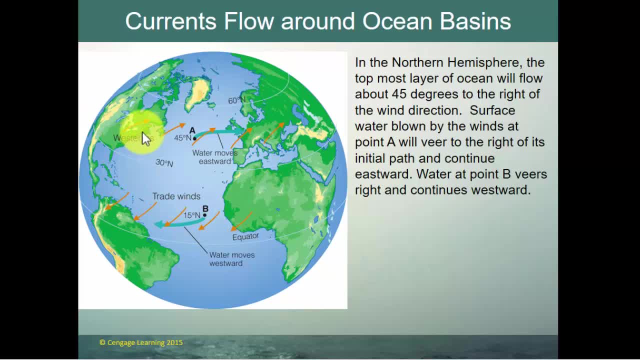 hemisphere, where coriolis will deflect the ocean current about 45 degrees to the right of the wind direction. Surface water blown by the winds will flow at about 45 degrees to the right of the wind direction. Surface water blown by the winds at point A will then veer to the right of the initial path and continue eastward. 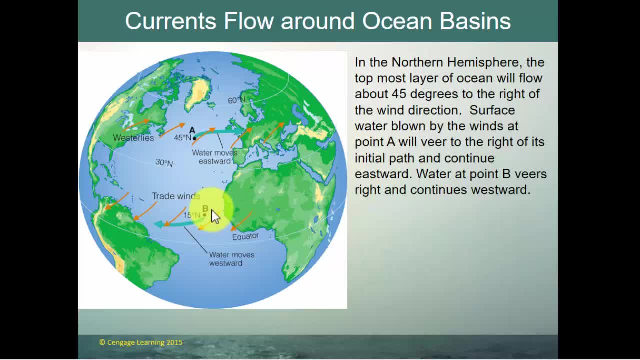 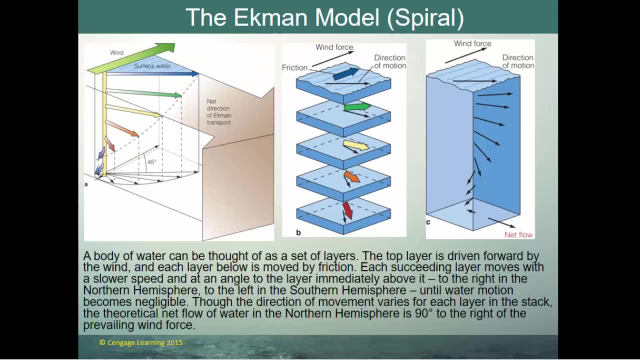 And then water at point B veers to the right- here's B and continues westward And again, creating that ocean gyre that we see in the major ocean basins, And this veering of 45 degrees is known as Ekman. 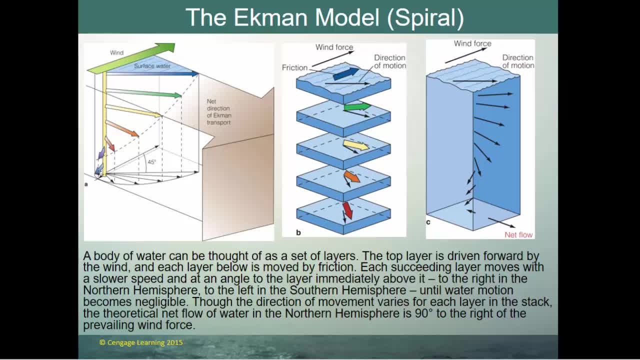 currents, or the Ekman model, or the Ekman spiral, depending on how you want to define it. So again, the wind at the surface is blowing in this direction and, because of coriolis, the surface water blows at about 45 degrees to the right of it, But each 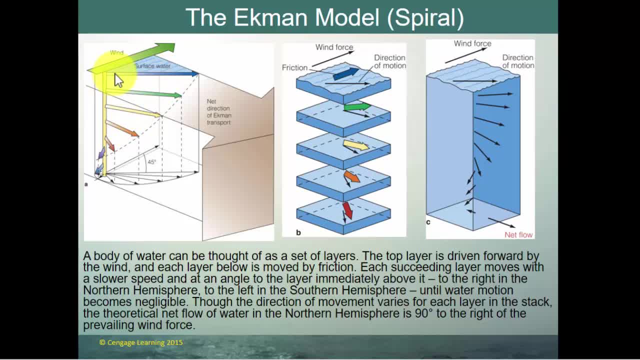 additional layer deeper and deeper in the water also blows to the right or moves to the right of the layer above it. So as you go deeper and deeper, those ocean currents continue to move to the right of the initial flow until you get to the very, very bottom. 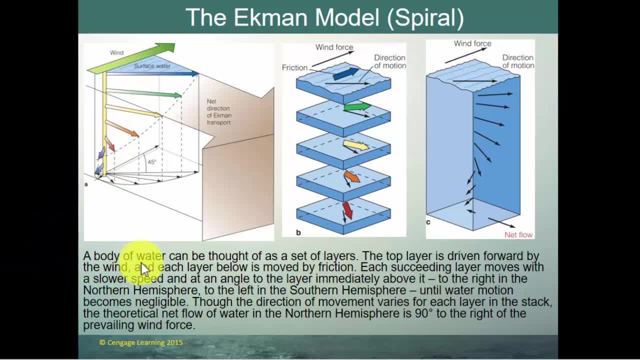 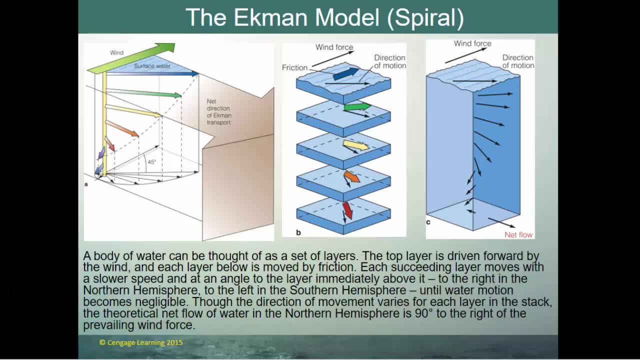 layer below is moved by friction. Each succeeding layer then moves with a slower speed and at an angle to the layer immediately above it, to the right in the northern hemisphere, to the left in the southern hemisphere, until water motion becomes almost negligible, Although the direction 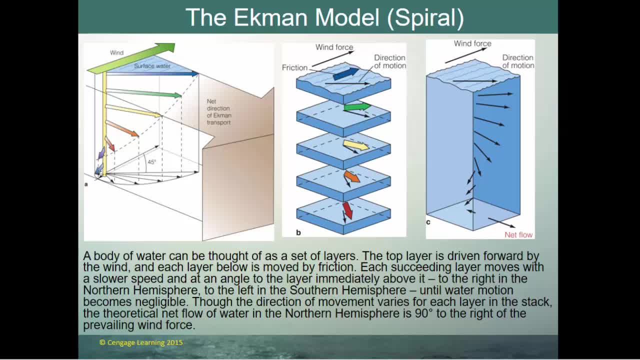 of movement varies with each layer in the stack. the theoretical net flow of the water in the northern hemisphere is about 90 degrees to the right of the prevailing wind. Now the previous slide. we talked about 45 degrees. That is going to be for the surface water. When you consider 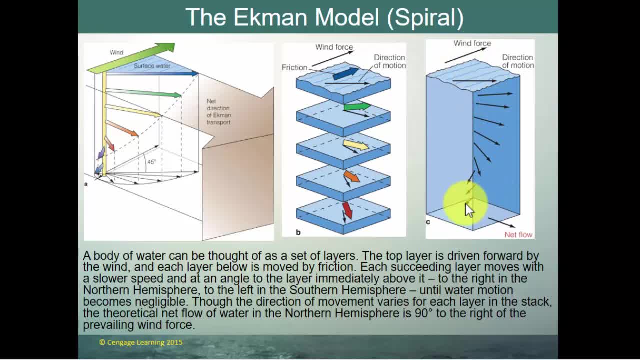 all the water movement in the entire deep layer in which the movement is affected, the net effect is about a 90 degree. So at the surface it's about a 45 degree flow, but the net effect is about a 90 degree flow to the actual wind motion. And again this is known as the Ekman spiral. 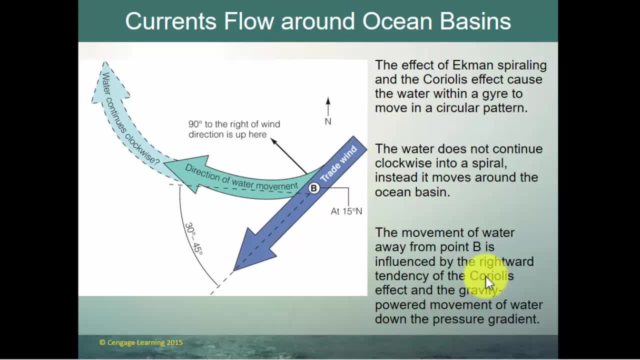 The effect of Ekman spiraling and the Coriolis effect caused the water within the gyre to move essentially to the right of the prevailing wind. So at the surface it's about a 45 degree flow, essentially in a circular pattern. This is the northeast trade wind. This is the water at point B. 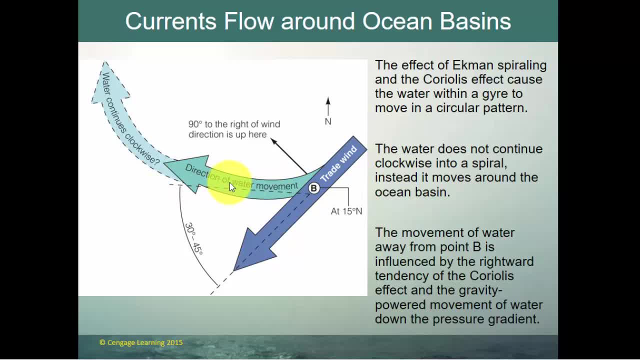 The direction of movement is about 45 degrees and then it continues to be deflected to the right and the water continues clockwise. It does not continue clockwise into a spiral, but instead generally moves in that circular motion around the basin: The movement of water away from point B. 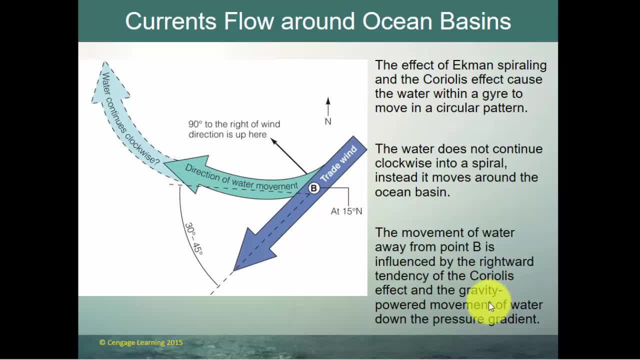 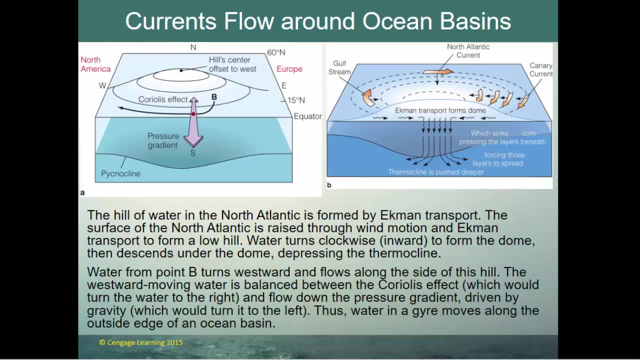 is influenced by the rightward tendency of the Coriolis effect and the gravity-powered movement of the water is influenced by the rightward tendency of the Coriolis effect. The movement of water down the pressure gradient, That gravity-powered movement of water down the 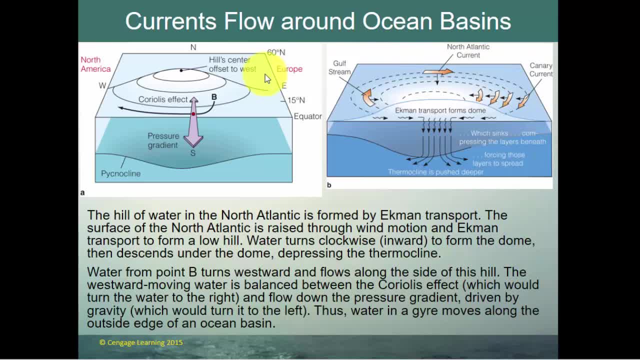 pressure gradient occurs because this Ekman spiraling causes water to pile up in the center of the gyre and so water wants to flow down that pile, downhill off that pile. There is a hill of water in each ocean basin. There's a hill of water in the North Atlantic. 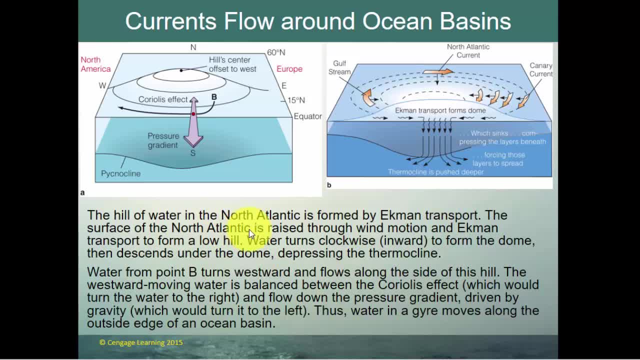 formed by the Ekman transport. The surface of the North Atlantic is raised through wind motion and Ekman transport to form a low hill, So water turns clockwise and inward from the dome, then descends under the dome, depressing the thermocline. So you can see it depresses down. 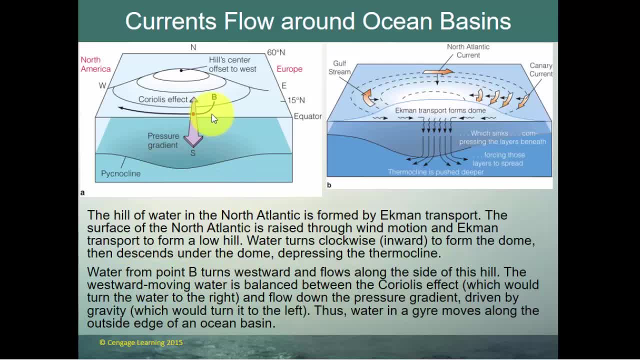 that thermocline Water movement from B turns westward and flows along the side of the hill. The westward moving water is balanced between the Coriolis effect, which would turn the water to the right, and the flow down the pressure gradient, which would want to cause it to go to the south. 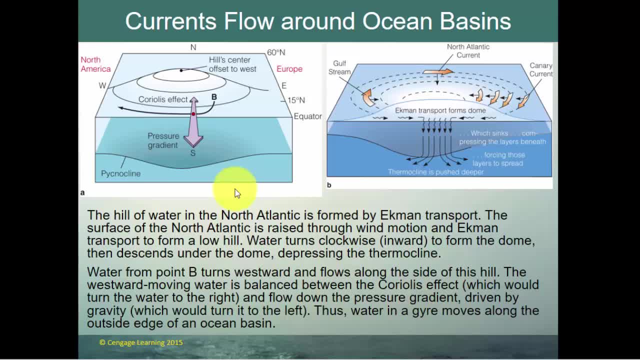 which is driven by gravity. Thus the water, in a gyre kind of, moves around the edge of the ocean basin. So it's a combination of the Ekman current turning it to the right, combined with this downhill movement turning it south, that just causes it to generally and gradually move in a clockwise flow around the ocean basin. 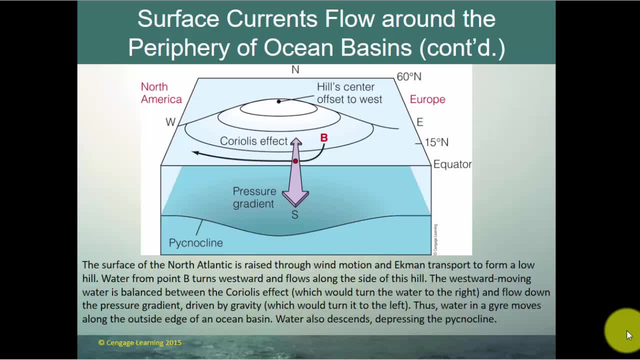 So another way to look at this surface current flowing around the periphery of the ocean basin. again, the water at point B is being blown from the north and east by the trade winds. That's one of the things that we want to look at. So we want to look at this surface current flowing around the 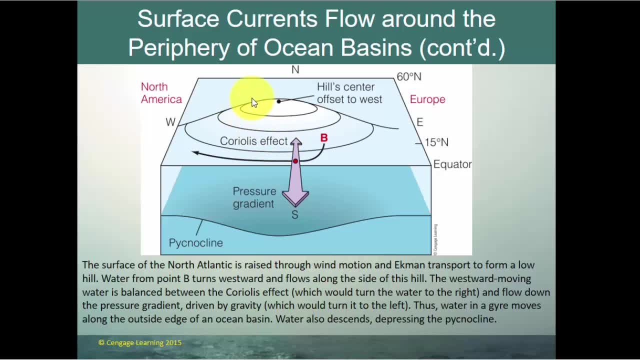 here at point W, now we want to look at this surface current flowing around the equator and we can get a sense of the depth and depth of the curve. So basically, here on the earth's morality, here on this earth's monetary estimate. 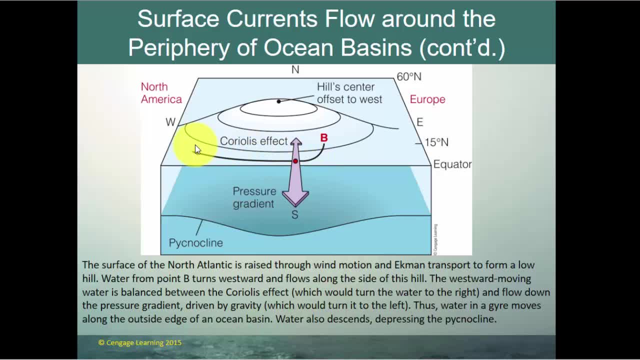 we want to look at this universoic°overlight Coriolis effect and the net effect of the water is to be deflected to the west and then basically around that ocean basin Now, because the Coriolis effect is stronger to the north than it is to the 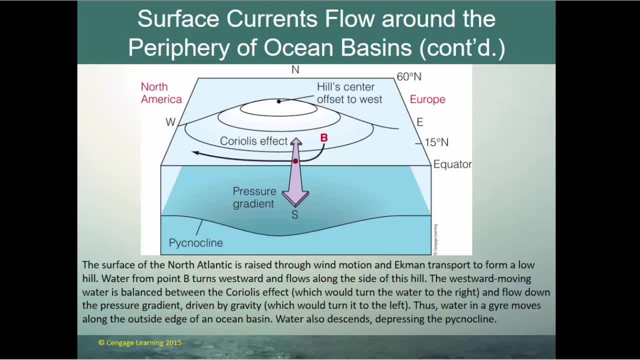 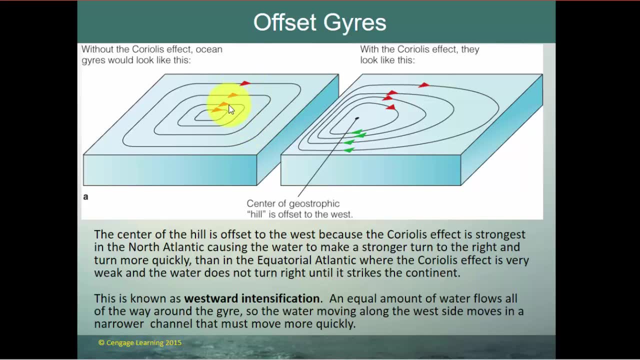 south, that hill is also offset to the west, And this is what that looks like in terms of the hill being offset to the west Without the Coriolis being stronger to the north than it is to the south. you'd have this nice round circle around the ocean basin. But because Coriolis increases, 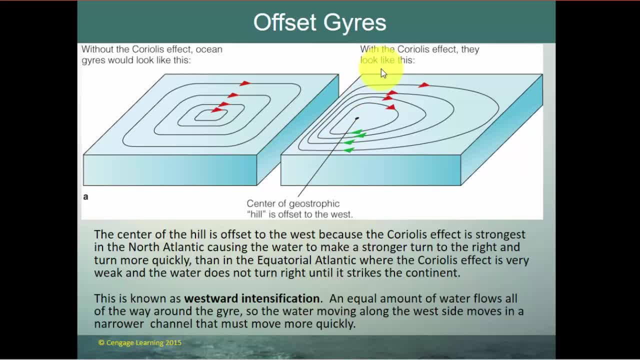 from the equator to the North Pole. the Coriolis effect is going to be stronger in the North Atlantic. Because it's stronger in the North Atlantic, the water is deflected in a greater force to the right in the North Atlantic, causing this quicker turn. So your North Atlantic flow. 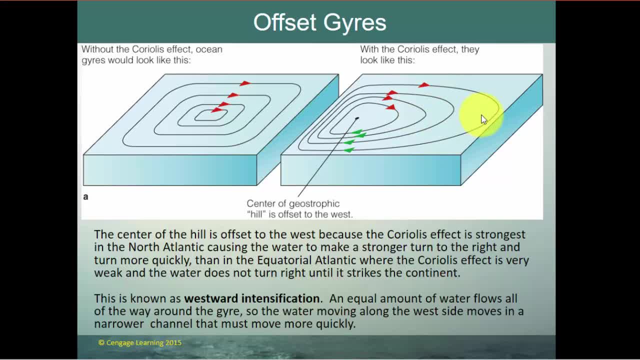 is a much broader flow. It is much wider across the eastern side of the Atlantic basin where, Whereas here, there is less of a turn to the north and the water gets sort of piled up along the edge of the basin. The effect of this: broader flow around the east side and a narrower flow around the west. 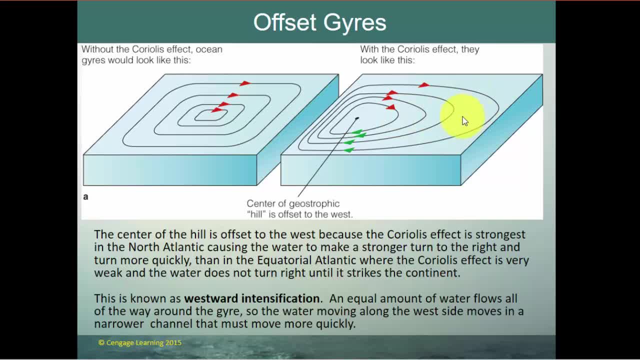 side. the water flowing in a broader channel essentially will move more slowly. The water flowing in a narrower channel will move more quickly, and this is known as western intensification. Without the Coriolis effect, the gyres will look like this: 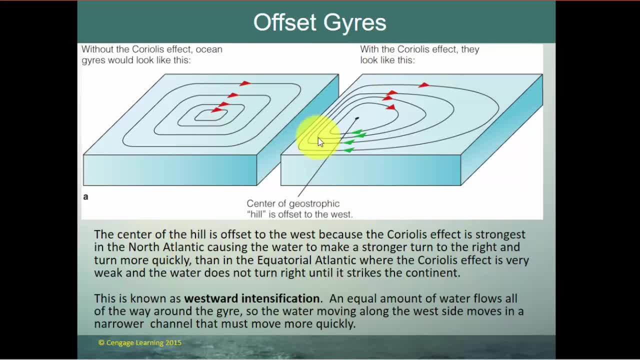 With the Coriolis effect and the fact that the Coriolis effect is strongest in the North Atlantic, it makes a stronger turn to the right and it turns more quickly than at the Equatorial Atlantic. So what ends up happening is you get this western intensification. 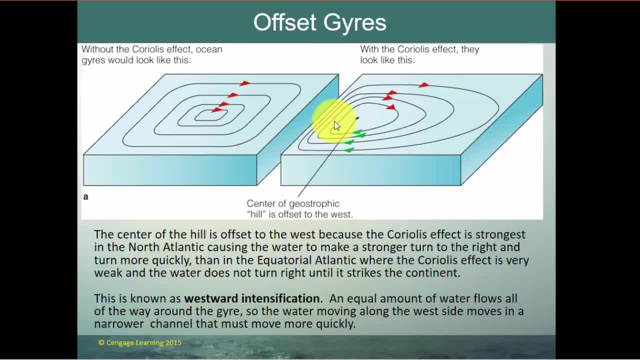 An equal amount of water flows all the way around the gyres, so the water has to move more quickly on the west side, in this narrower channel, than in the broader channel on the east side, And that is known as westward intensification. And again, here's another look: a cross-section of the flow in the North Atlantic, known as. 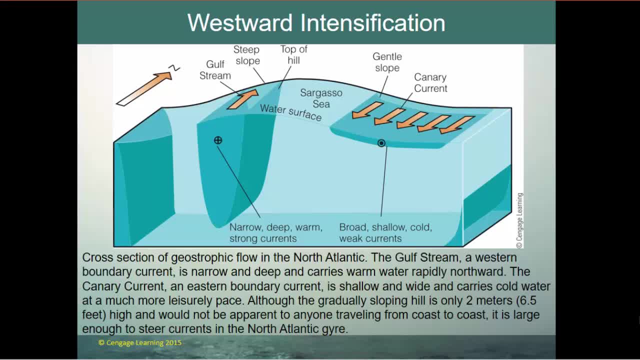 the geostrophic flow, Which is the most important one. It's a model flow. The Gulf Stream is a western boundary current, so the Gulf Stream is on the west side of our mound, on the west side of the basin. It is a western boundary current, it's on the west side of the basin. 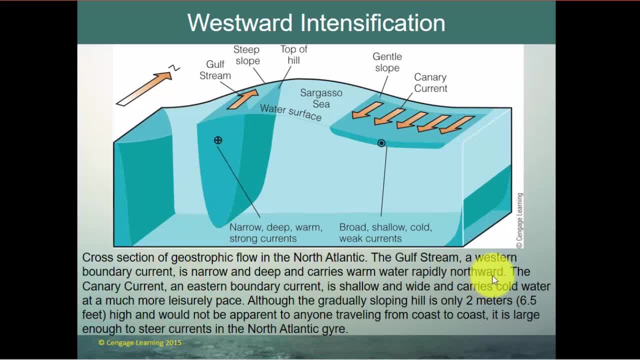 It's narrow and it's deep and it carries warm water very rapidly to the north. The Canary Current is on the east side of the basin and the east side of the slope it is a broader, wider slope, so it's much shallower. 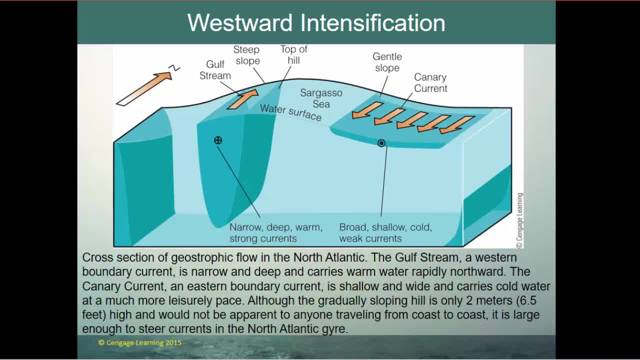 It's an eastern boundary current, a shallower current, a wider current that carries more cold water at a much more leisurely pace to the south. Although this gradually sloping hill is only about six, six and a half feet high, it really. 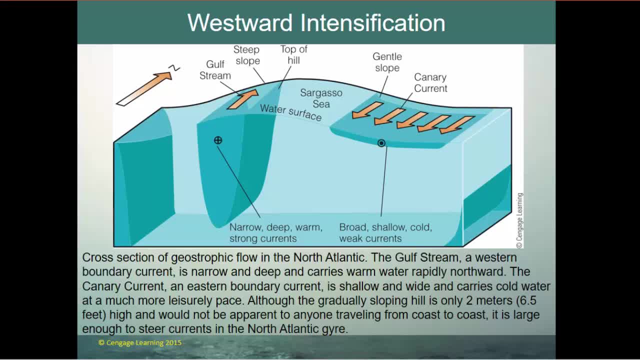 wouldn't be apparent to anyone traveling from coast to coast. It is large enough to help steer the gyres in each basin, in this case the North Atlantic Gyre. So what does this look like? The surface currents around the ocean basin. 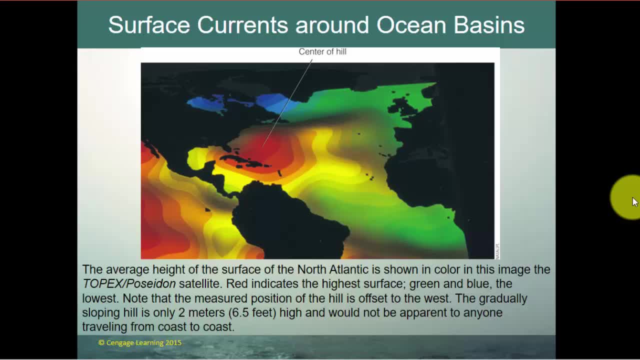 Two things are going to happen due to western intensification: 1. Warm water flowing up the west side of the basin and cool water flowing down the east side of the basin in the northern hemisphere. That's one thing that's going to happen, and really three things. 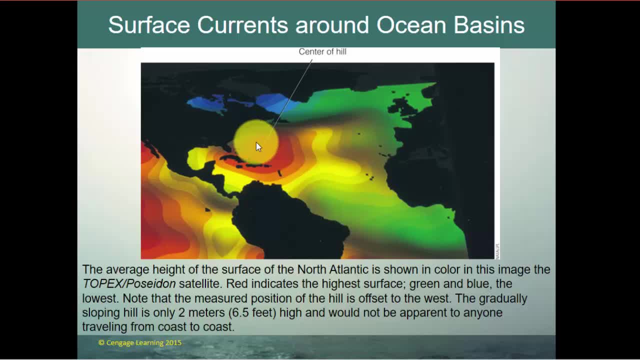 The second thing is going to be: the western boundary current is going to be narrow and stronger, The eastern boundary current is going to be weaker and that hill we talked about in the center of the Atlantic Ocean is offset to the west. The actual hill is going to be offset to the west. 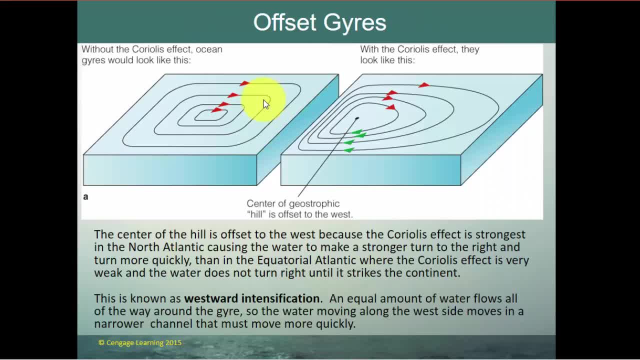 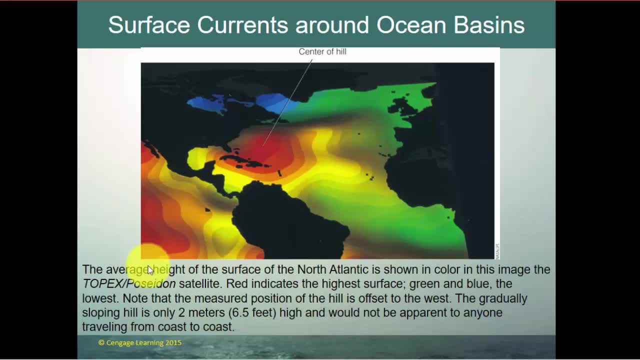 If we look back here, the hill is offset away closer to the western boundary, current 2.. We see that here as well, with the center of the geostrophic hill being offset to the west. The average height of the surface of the North Atlantic is shown in color in this image from. 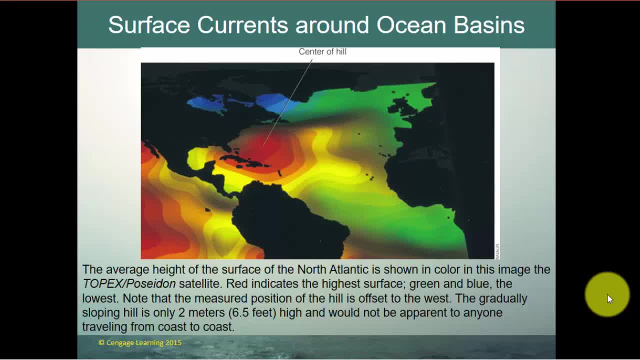 the Topaz Poseidon satellite. Red indicates the highest surface, green and blue the lowest. You can see that this hill is offset to the west with the western boundary current, the western intensification. Really, this hill is only about 2 meters or about 6, 6.5 feet above the surface, so you 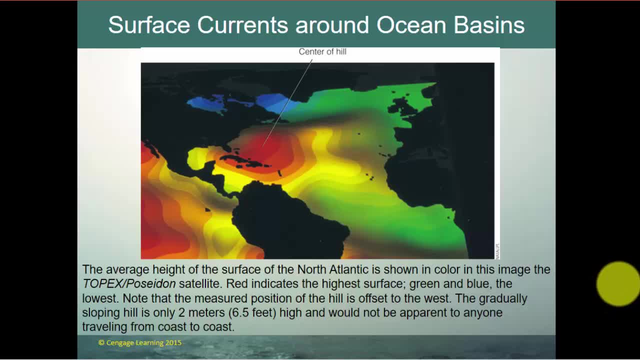 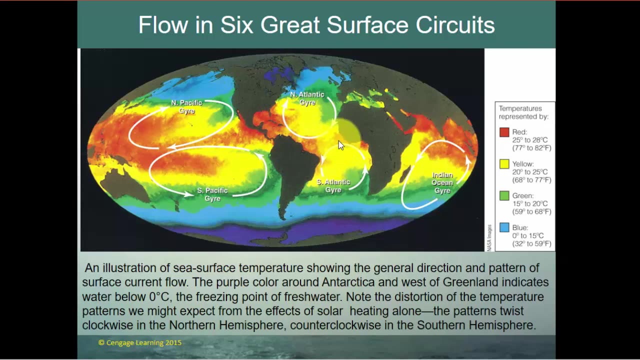 really wouldn't notice it. It's not a mountain across the Atlantic Ocean, but it's enough of a hill to cause that gyre to go very much around the Atlantic Ocean in a circle. Alright, there are six great gyres. There is the North Atlantic Gyre, which we talked a lot about, the South Atlantic Gyre. 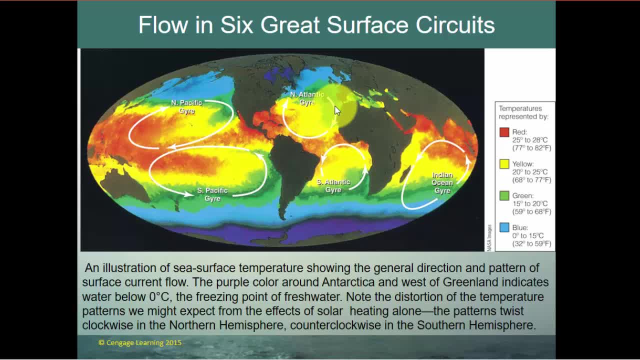 North Pacific, South Pacific and then the Indian Ocean, Gyre. You can see how the west side of the northern hemisphere carries warm water north, because we're looking at here our sea surface temperatures 3. Here's the North Atlantic, the Canary Current, bringing cool water south. 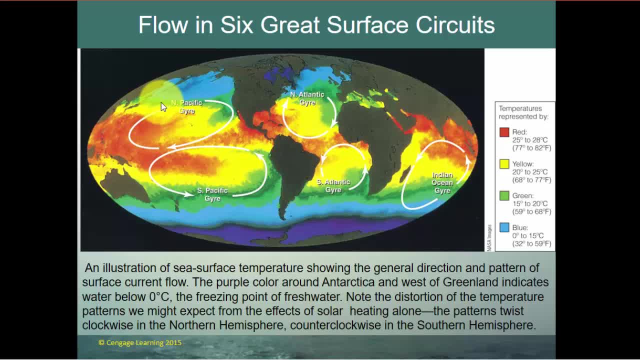 In the Pacific Ocean you've got the Corotio Current carrying warm water north and then the California Current carrying cold water south. Here you have in the southern hemisphere it's the opposite, where warm water is traveling toward the poles here and cool water is traveling toward the equator here. 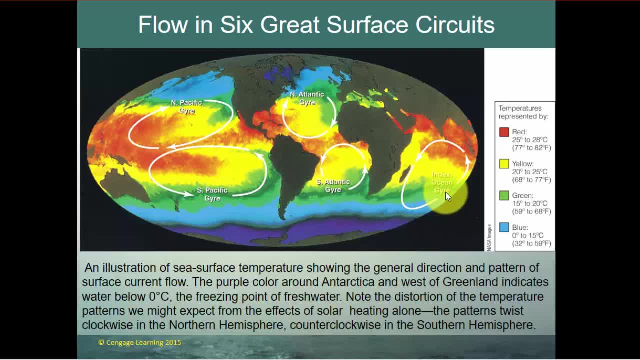 Same thing in the South Atlantic: warm water is moving south, cool water is moving north. And then in the Indian Ocean you have that warm water moving south and cool water moving to the north. This is an illustration of sea surface temperatures, not the heights like the previous slide, but 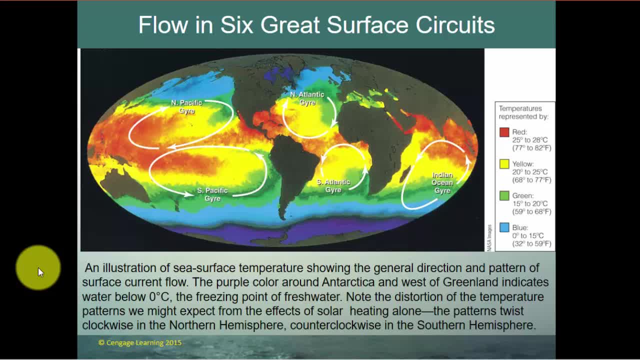 temperatures, showing the general direction and pattern of the surface current flow. The purple color around Antarctica and west of Greenland indicates water below zero Celsius, the freezing point of freshwater. Note that the distortion of the temperature patterns that we would expect from the effects of solar heating alone, that is just warm at the equator, that warm water is twisted. 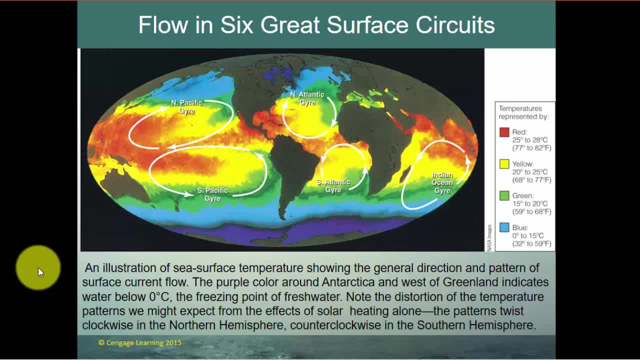 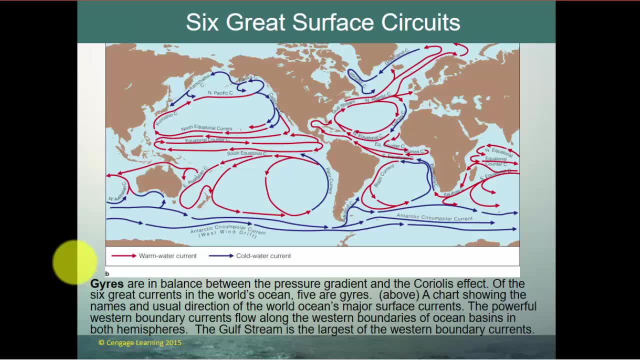 northward in the northern hemisphere. This is what the six great currents look like and of course, the arrows indicate the temperature of the water: The Corotio Current carrying warm water north. the California Current carrying cool water south Gulf Stream warm water north and the North Atlantic taking that water all the 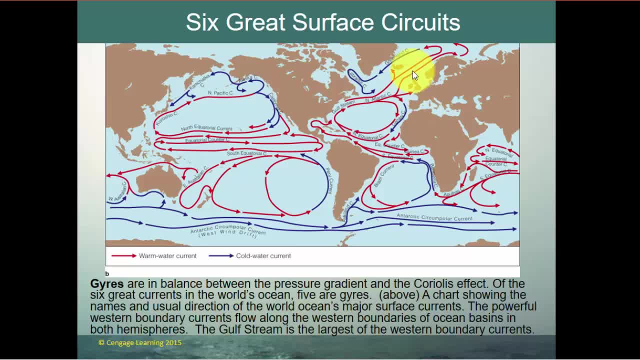 way over to Western Europe, And this is the reason why Western Europe- it may be chilly up there at times but it's not nearly as cold As the land mass is at the same latitude over North America because it has that warm ocean current carrying warm ocean water and air to that region. 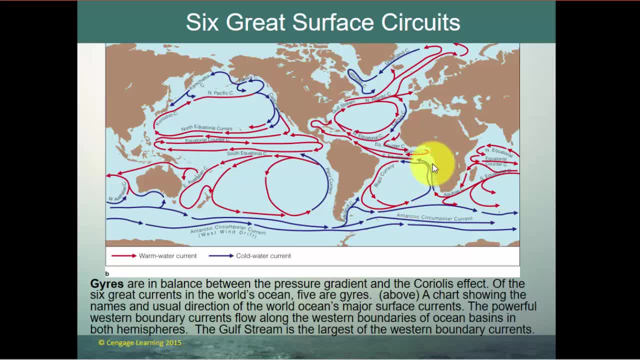 Again. the Bangla Current in South Africa is carrying cold water to the equator. The Brazil Current is carrying warm water south. The East Australian Current is carrying warm water south. The Peruvian Current is carrying cold water north. There's the Corotio and the California, as we said. 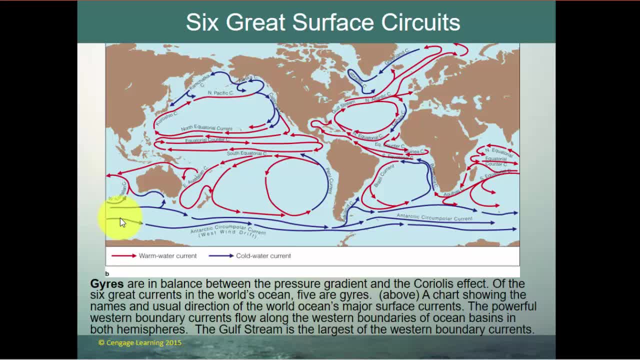 And then There's one last major current in the ocean, and that's the Antarctic Circumpolar Current, also known as the West Drift. It travels westward around the entire globe. There's no land mass to deflect it, so it just travels around the globe. 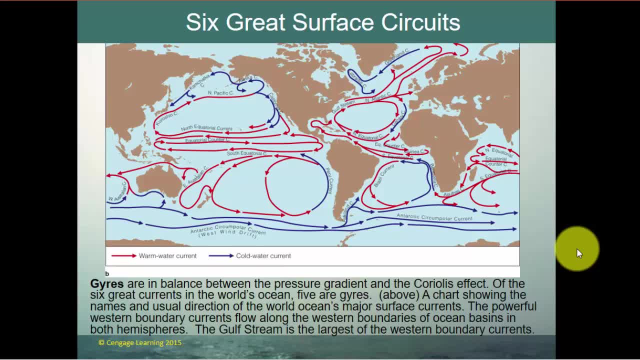 So gyres are in balance between the pressure gradient- that's, the pressure gradient going down the hill- and the Coriolis Effect. The pressure gradient wants to carry the water down the hill, The Coriolis Effect wants to turn it to the right. in the northern hemisphere, the left. 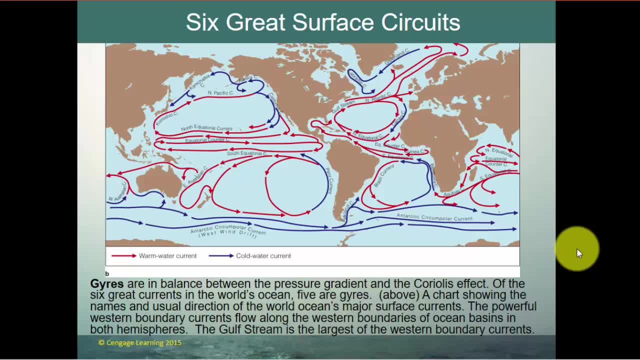 in the southern hemisphere And the effect is the gyre. So the graph shows the power of the six great ocean currents, five are gyres And this chart shows the names and the usual direction of those major ocean currents And you can see the powerful Western Boundary Currents flow in the west boundaries of the 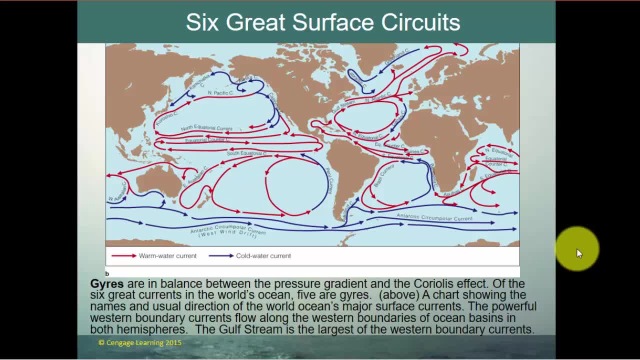 ocean basin and the Eastern Boundary Currents in the east side of the ocean basins. And the Gulf Stream is the largest and most powerful current in the world and largest and most powerful Western Boundary Current as well. All right, So Western Boundary Currents. 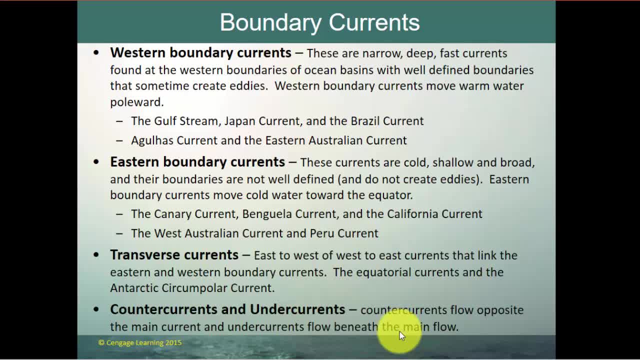 These are the narrowest deep and fast currents found on the western borders of ocean basins with well-defined boundaries that sometimes create actual eddies. Western boundary currents show move. that is warm water poleward. It's the Gulf Stream, the Japan Crocio Current and the Brazilian Current. 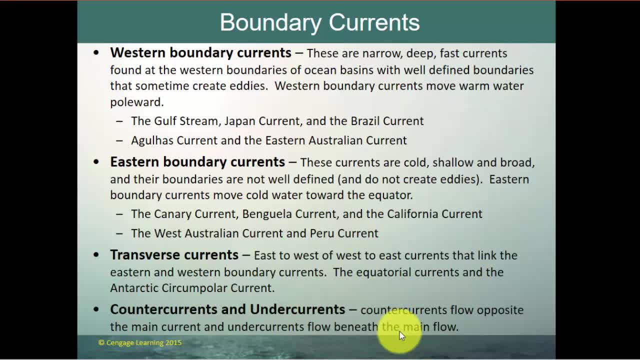 And we also have eastern boundary currents. These currents are cold, shallow and broad and their boundaries are not very well-defined. They do not create eddies, And eastern boundary currents move cold water toward the equator, like the Canary, the Bangalore and the California. 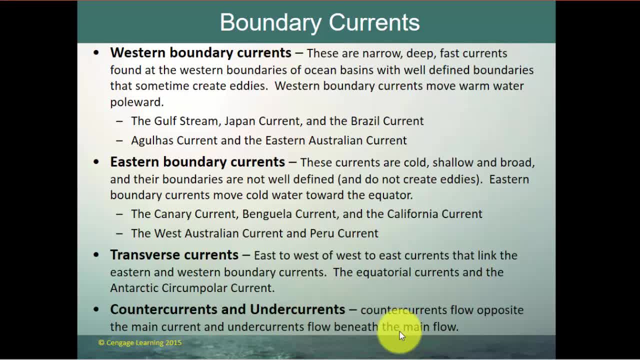 Current Transverse currents, that is, move east to west and west to east, and they link the eastern and western boundary currents. So to complete that, Gaia, you have to have something that links the eastern boundary and the western boundary currents, and those are those transverse currents. 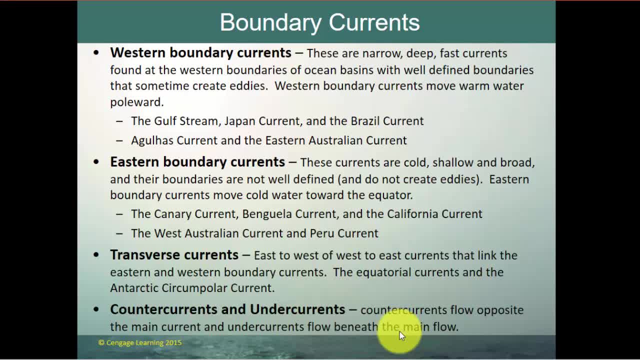 So the equatorial currents and the Antarctic circumpolar currents are the transverse currents, And then you have countercurrents and undercurrents, and countercurrents will flow opposite to the main current and undercurrents will flow beneath the main flow and they may be flowing. 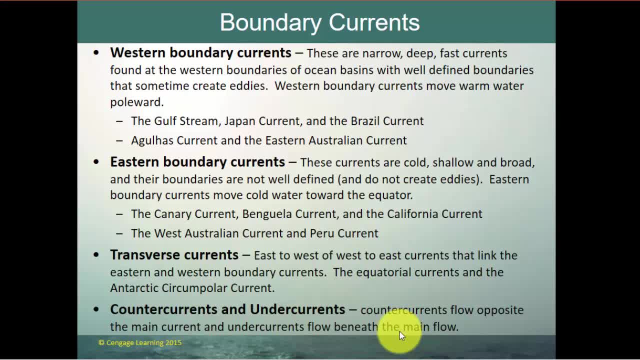 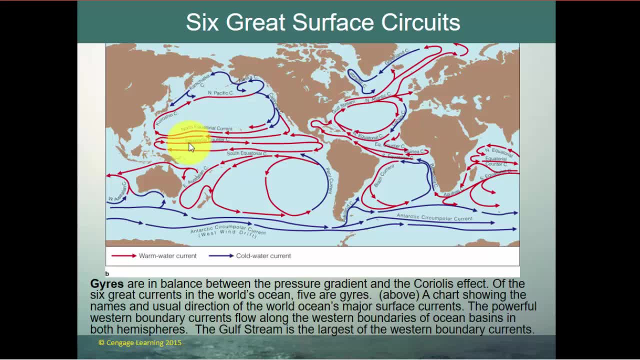 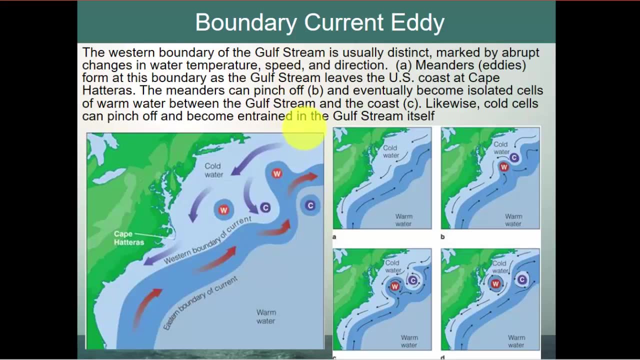 with the flow or counter to the main flow, And here we have the equatorial current, which is going to be a countercurrent. That's one example of that. All right, we mentioned when we were talking about western boundary currents that sometimes 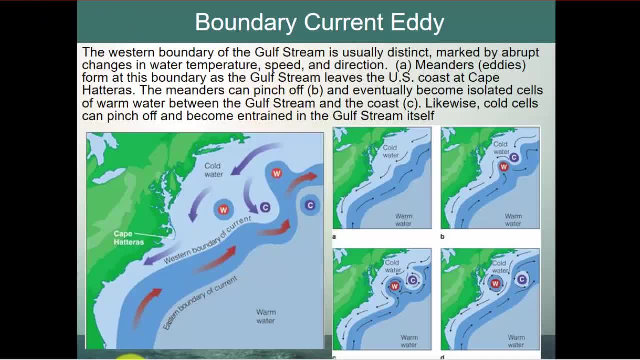 they create a flow, And so we're going to talk about that in a little bit, And then we're going to talk about the eddies, and this is what those eddies look like. where this western boundary current in the North Atlantic is the strong Gulf Stream and there's 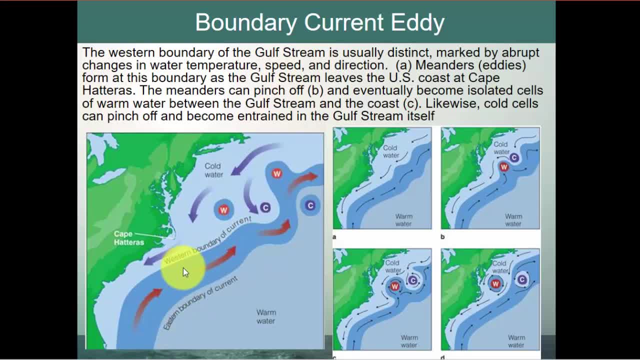 the west side of the current and the east side of the current. Both are very, very well defined And as that water moves north, the cold water that's moving back down to the south sometimes gets entrained into that western boundary current and it creates these eddies. 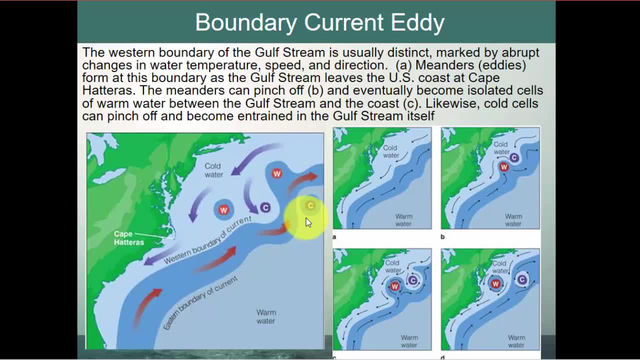 where warm water will spin off and cold water will get pulled in. And so you start with the typical cold current moving south, the warm current moving north, and then some of that cold water gets entrained and so you get a little pool of warm water that gets. 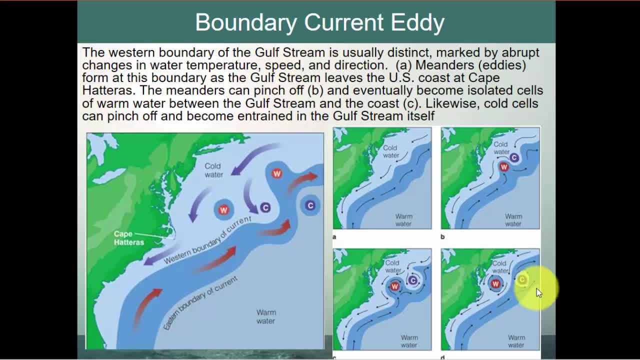 displaced and that cold water gets pulled into the actual current and sometimes it then gets ejected out of the eastern boundary of the current. So the western boundary of the Gulf Stream is usually distinct and marked by abrupt changes in water temperature, speed and direction. Meanders or these eddies will form as the Gulf Stream leaves the US. 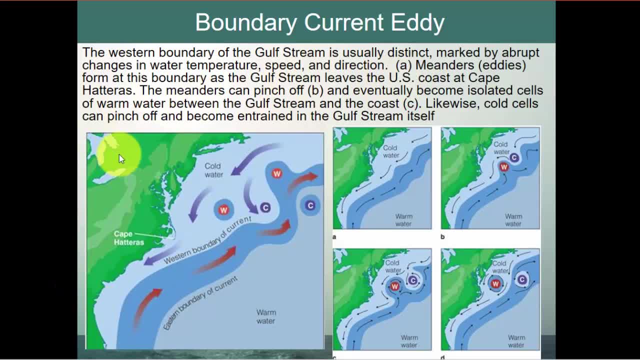 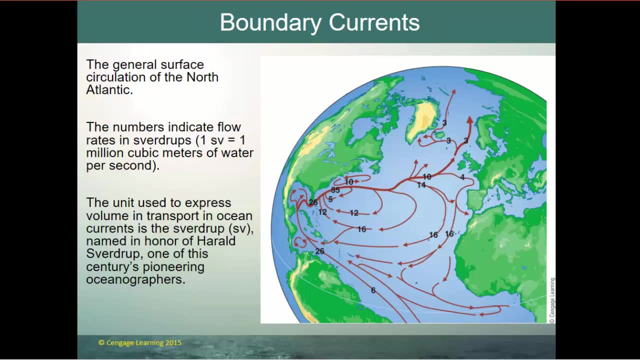 coast at about Cape Havoc. The meander can pinch off and eventually become isolated cells of warm water between the Gulf Stream and the coast. Likewise, cold cells can pinch off and become entrained in the Gulf Stream itself, The general surface circulation of the North Atlantic. So the numbers indicate the flow. 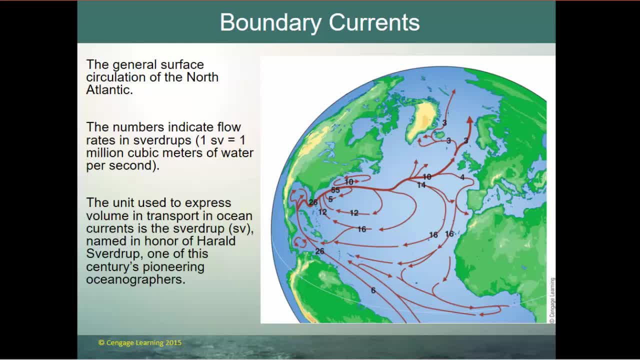 rates and these- this very odd Swedish word S-V-E-R-D-R-U-P-S- the spherdrups. So one spherdrup equals one million cubic meters of water per second, and you can see that the Gulf Stream. 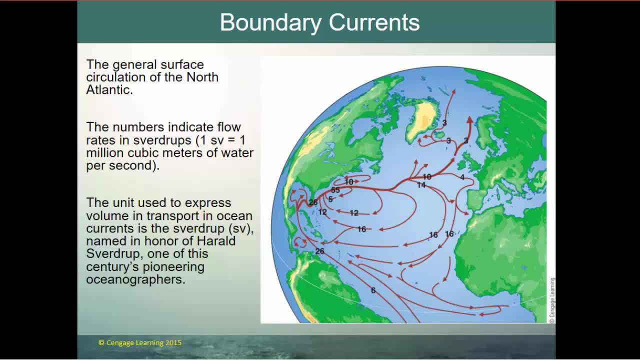 is 26 to 55 million cubic meters of water per second. So the spherdrup again, that's that. that word S-V-E-R-D-R-U-P-S moves a tremendous amount of water in the Gulf Stream. 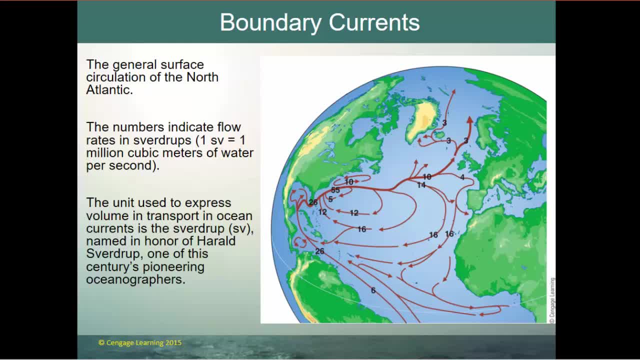 and you can see there's a lesser amount of water in different currents. The unit is used to express the volume and transport in ocean currents and it's named and it's called S-V-E-R-D-R-U-P-S. S-V-E-R-D-R-U-P-S. 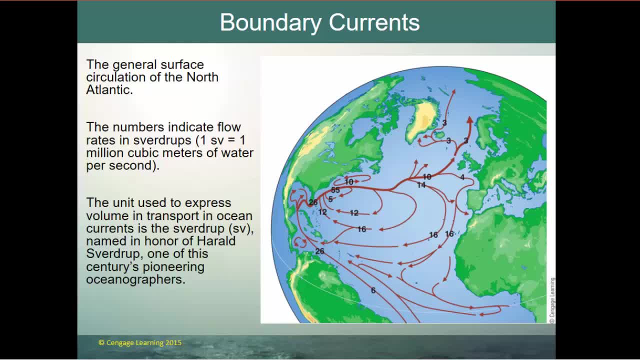 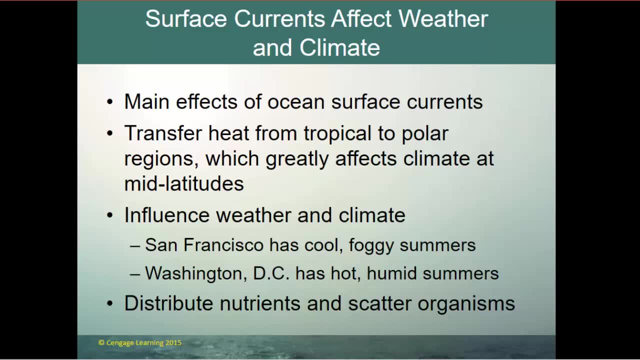 S-V-E-R-D-R-U-P-S. S-V-E-R-D-R-U-P-S. It's named in honor of this herald, who was one of the century's pioneering oceanographers. The main effect of ocean currents is to transfer heat from the tropical regions to the polar regions. 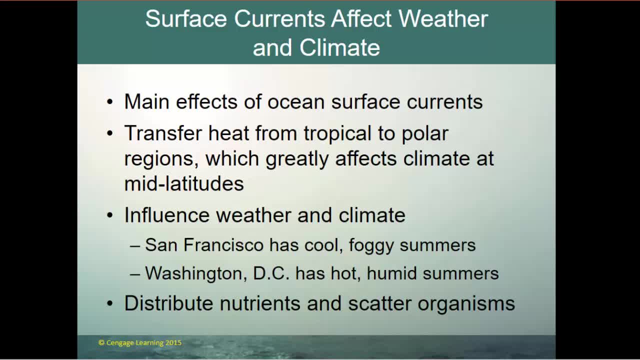 which generally and greatly affects climate. at the mid-latitudes. The influence on weather and climate can be seen because San Diego has those cool, foggy summers. Mark Twain once said the coldest winter he ever spent was one summer in San Francisco. 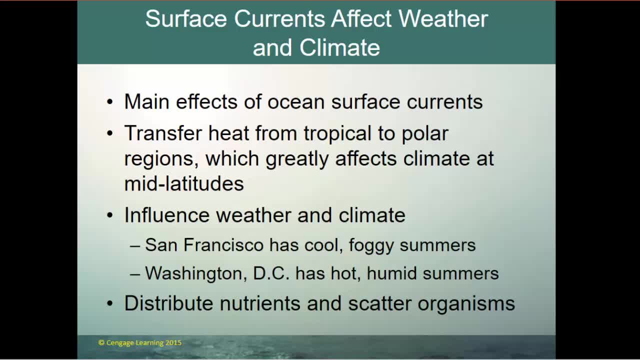 And, of course, Washington DC has hot, humid summers because of the Gulf Stream that moves just by it. So the two influences, the two main impacts of ocean currents are to transfer heat from the tropical to the polar regions and also to distribute nutrients and scatter organisms around the ocean. 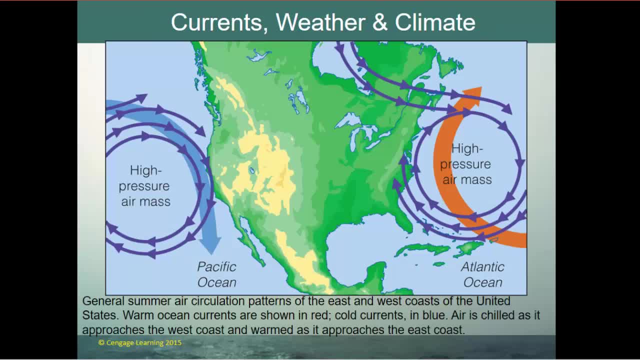 So we talked about San Francisco being cold. The Big Gyre in the North Atlantic moves that cold northern Pacific water south in the California, The California Current, that eastern boundary current keeping California nice and cold, Where the Atlantic Gyre, the North Atlantic Gyre, brings warm, moist water north with the Gulf Stream. 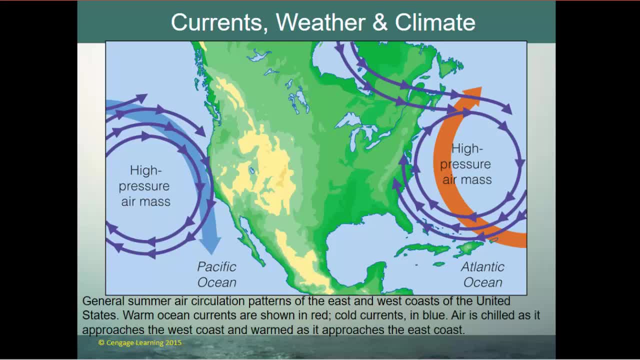 keeping the eastern seaboard very warm. So these are generally the summer air circulation patterns on the east and west coast of the United States, And warm ocean currents are shown in red, The colder ocean currents are shown in blue, And air is chill as it approaches the west coast and warm as it approaches the east coast. 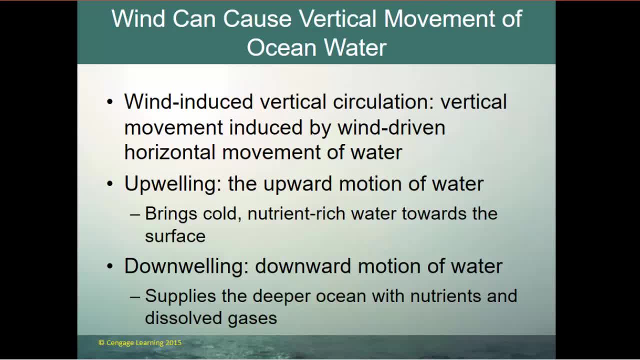 Wind can also cause vertical movements. So we talked an awful lot now in the last few minutes over how wind induces horizontal movements or these gyres or the ocean currents. But wind can also induce vertical circulations, the vertical movement induced by wind-driven horizontal movement of water. 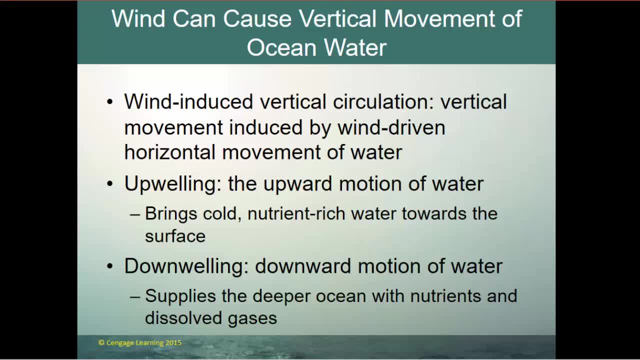 So, as the water moves horizontally across the ocean because of the wind, it can create either upwelling or downwelling. And upwelling is the upward motion of water- It brings cold, nutrient-rich water towards the ocean- And downwelling is the downward motion of water. 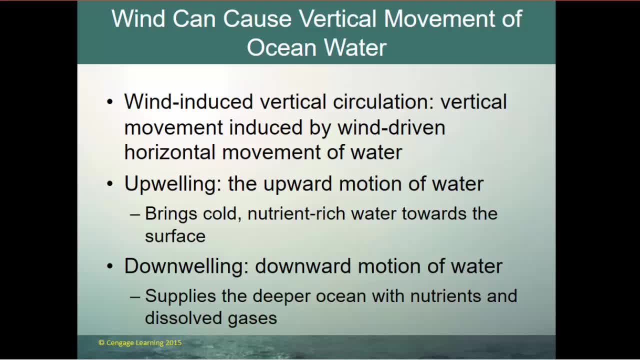 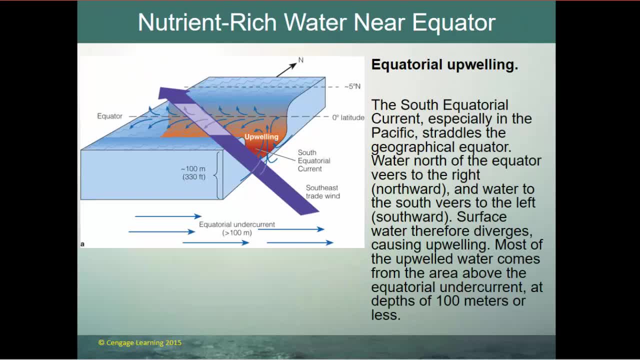 which supplies the deeper ocean with dissolved gases and nutrients. So this is what equatorial upwelling might look like. The south equatorial current, especially in the Pacific straddles, the geographic equator Water north of the equator veers to the right, northward. 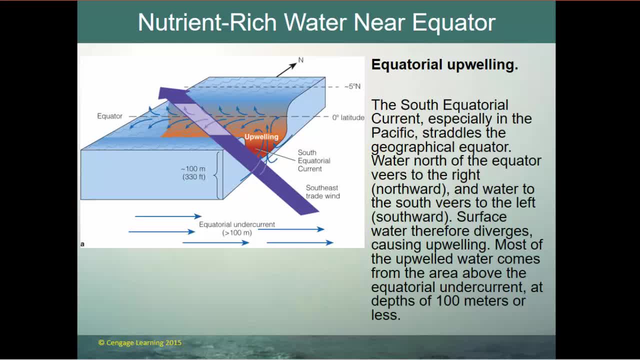 and water south of the equator veers to the left. That means the surface water diverges. So if you look right at that zero degree latitude right in here to the north, it moves to the north, to the right, to the south. it moves to the south, to the left. 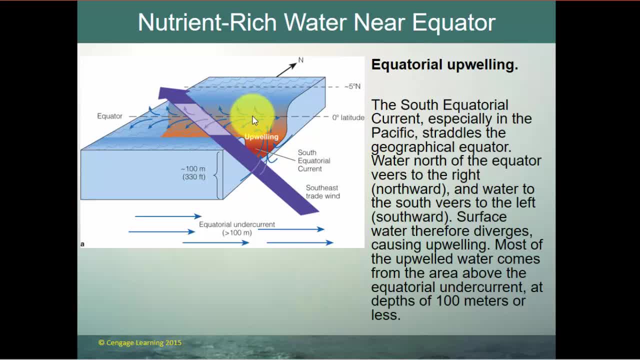 So the water here is diverging Water, the mass here is moving away, So it has to be replaced, And it's replaced by this upwelling. this upwelling, Surface water therefore diverges, causing upwelling. 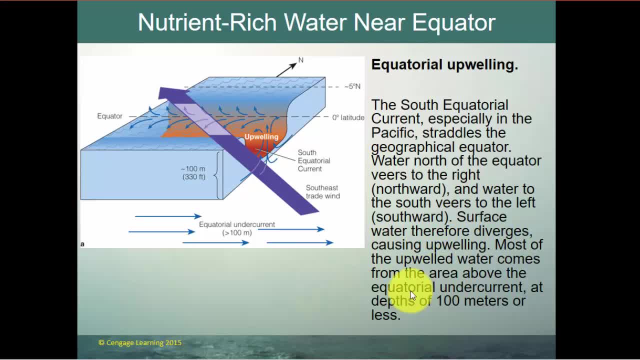 Most of the upwelled water comes from the air. Most of the water comes from the area above the equatorial undercurrent, at about a depth of 100 meters or so, So it brings this water upwards. So that's one example of how horizontal movement of water. 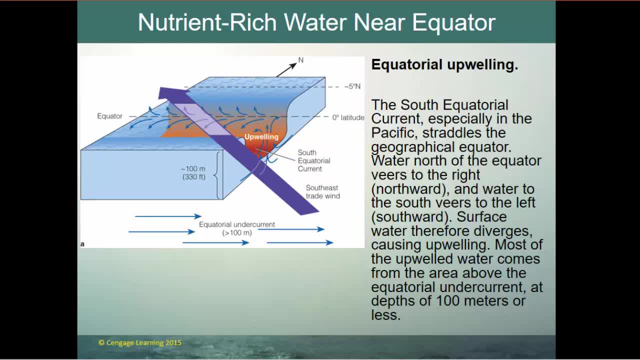 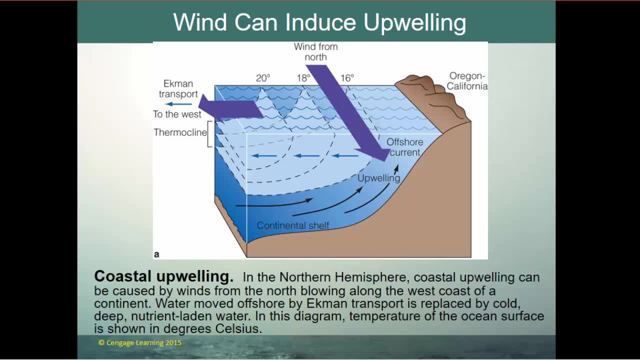 at the surface caused by wind creates a vertical movement of water at the surface And this is another way that wind can induce upwelling. We'll talk about the California current And wind from the north and along that California current blows north to south. 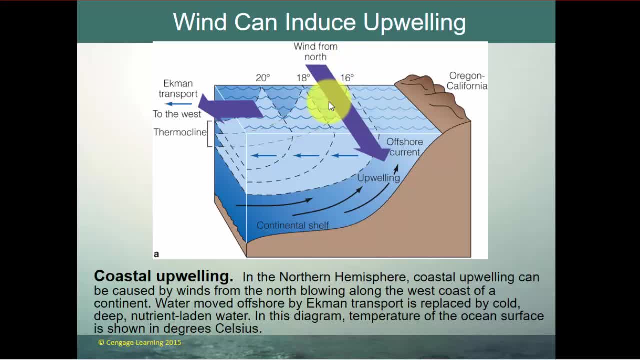 It blows north to south. Well, Ekman transport turns it to the right, And as it turns it to the right, it pulls all this water here offshore. And because it's moving all this water offshore, that water has to be replaced. 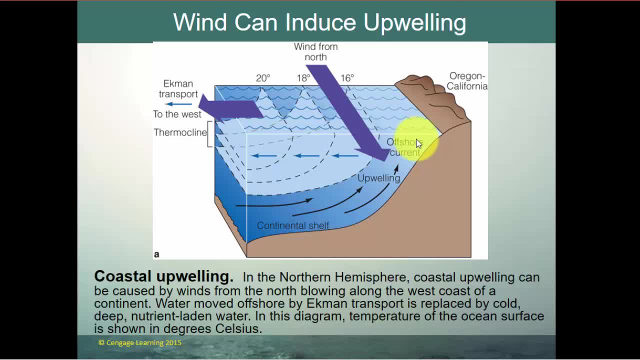 So it's replaced from deep below, creating upwelling. So that's coastal upwelling In the northern hemisphere. coastal upwelling can be caused by winds from the north blowing along the west coast of the continent. Water is moved offshore by Ekman transport and is replaced. 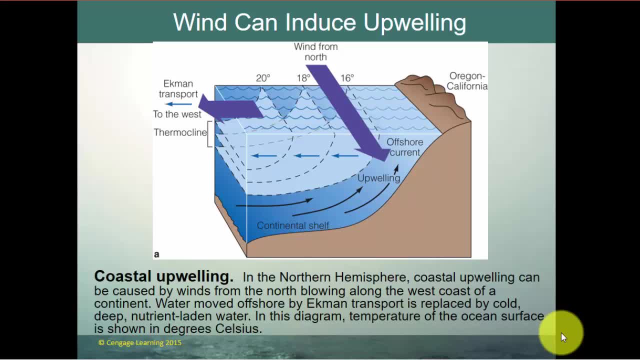 by cold, deep, nutrient-laden water. In this diagram, the temperature of the ocean surface is shown in degrees Celsius, And so what's very important about this is, off the coast of California, that Ekman transport, or that offshore movement of water. 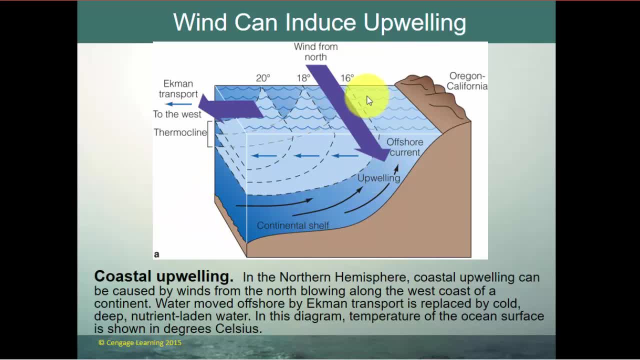 brings very cold, nutrient-rich water up along the coast of California, And that's why California is well known for its not only its kelp beds, but its small baitfish, its sardines and its smelt and its grunion and different types of fish, because they come to the surface. 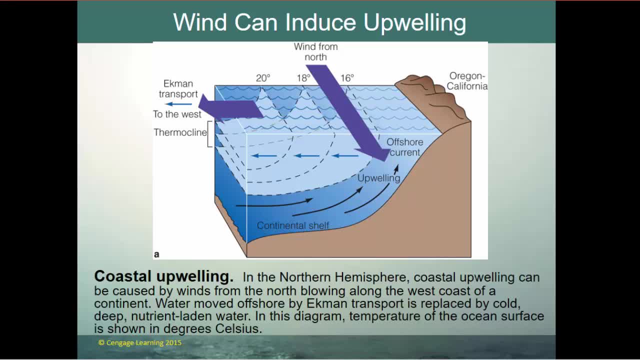 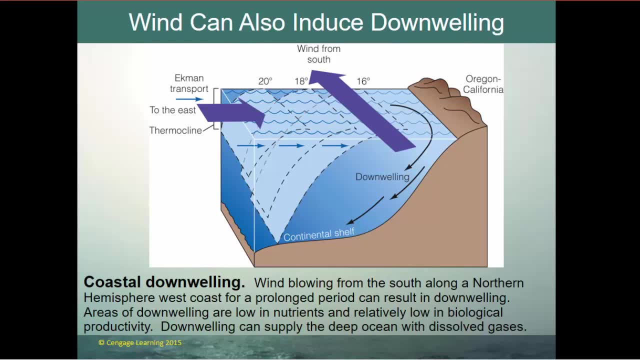 because all that nutrient-rich water is there And of course that feeds larger and larger fish. All right, You can also get. downwelling can also occur. So if the wind is blowing south along the northern hemisphere, west coast for a long period of time, so a south wind. 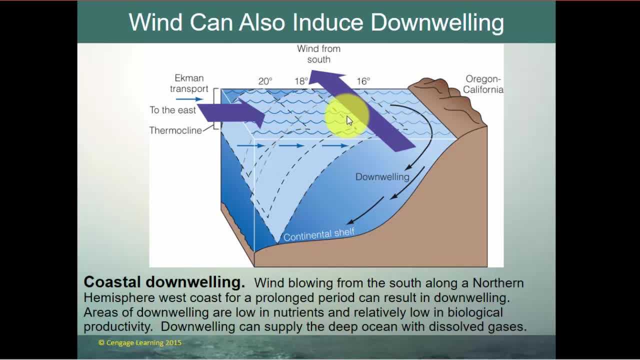 you're going to get the water moving northward and therefore turning to the right, And that's going to pull water off the Atlantic or onshore. When it hits the coast it goes down, So areas of downwelling. that's going to be warmer water. 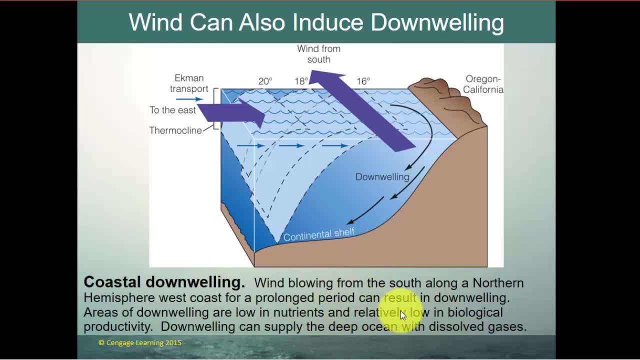 will be low in nutrients and relatively low in nutrient and biological activity at all, But it can supply the ocean with dissolved gases, meaning there's a lot of ocean-atmosphere interaction where oxygen, carbon dioxide, nitrogen will dissolve into the surface of the ocean. 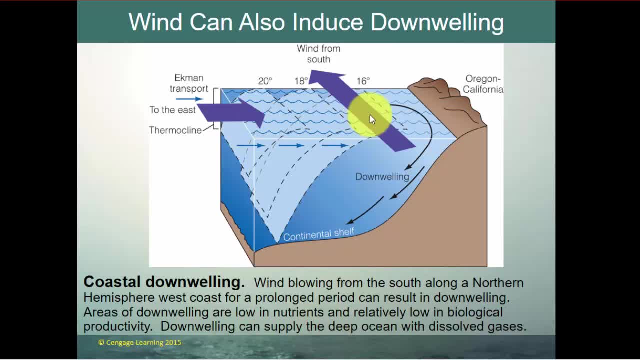 And if this south wind creates a right turn because of Ekman current or Ekman transport, it pulls water off the ocean. It pulls water onshore and forces water down So that warmer water at the surface gets forced down, taking dissolved gases below. 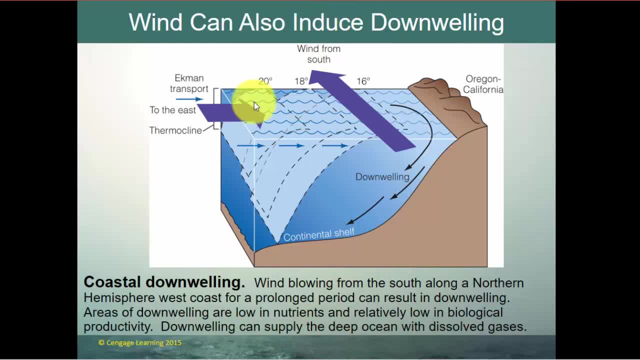 So again, a south wind creating a south current, Ekman transport forcing water toward the coast, and then downwelling occur. So winds creating horizontal movement of water, creating vertical movement of water. All right, So we're going to talk a little bit about what's known as El Niño. 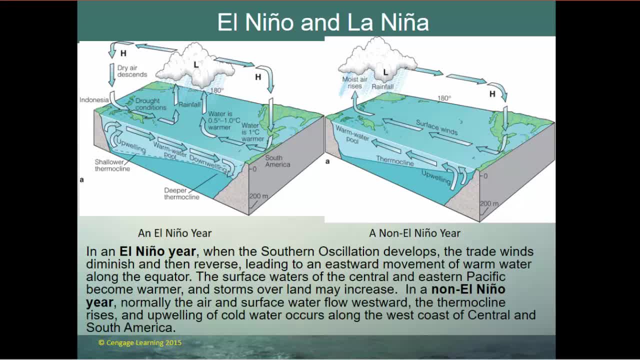 And of course there's also La Niña. But I'll tell you right off the bat, La Niña is kind of a um, something the media created. Really, what we have is El Niño and then non-El Niño years. 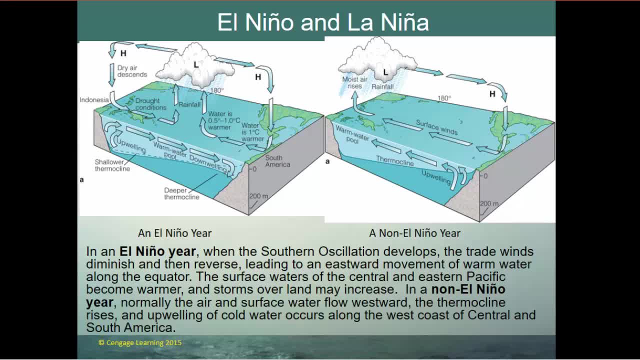 And the El Niño is tied to something called the Southern Oscillation. So sometimes El Niño is known as ENSO, which is El Niño E-N-S-O. Southern Oscillation. So what we're looking at is a non-El Niño year. 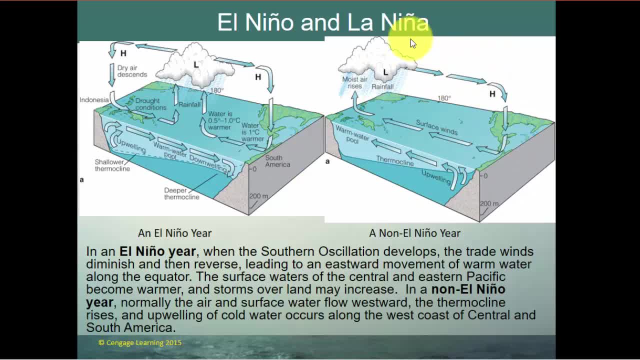 So this is this on the right-hand side is the normal situation across the Pacific Ocean. So what you're looking at is the Pacific Equatorial Regions And in the Pacific Equatorial Regions, because we have a northeast trade wind and a southeast trade wind, 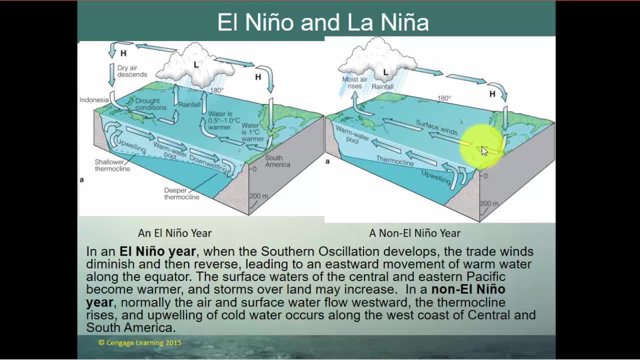 that equatorial transverse current moves from east to west. It moves from east to west, And so what that causes is air to rise off the surface in the west- because you get nice warm water over here- and sink toward the surface back in the east. 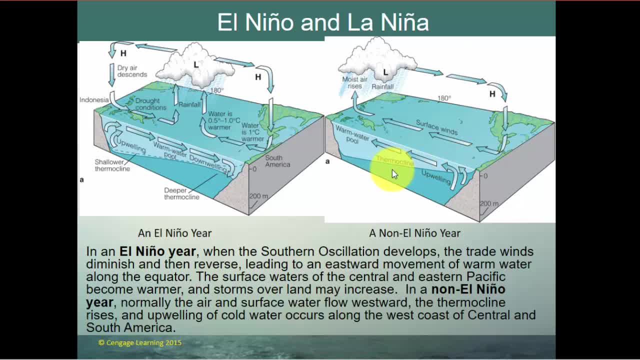 because you're going to have colder water here. Remember, cold water is brought in from the north, from the south, that is, with the Peru Current. California Current brings cold water in from the north here. Cold water, the air sinks over that cold water. 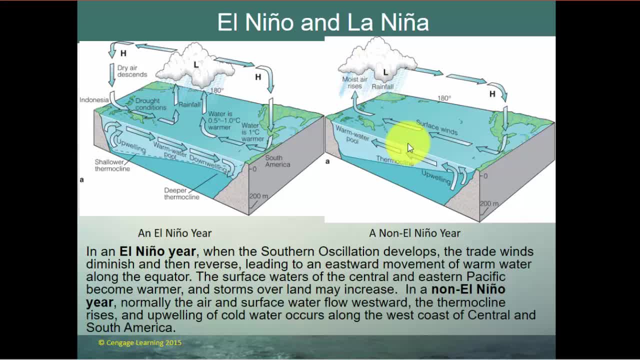 Warm water. here, air rises over that warm water, And so the typical non-El Niño year has a lot of warm water piled up on the west side of the Pacific Ocean and cloudy, wet weather where we have dry weather on the east side. 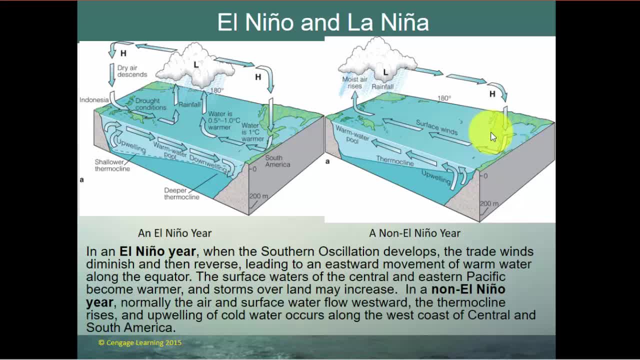 In an El Niño year, that is, the southern oscillation occurs, meaning the pressure patterns this low here and this high here. they flip And you get a little bit of a difference with the low forming sort of in the middle of the Pacific Ocean. 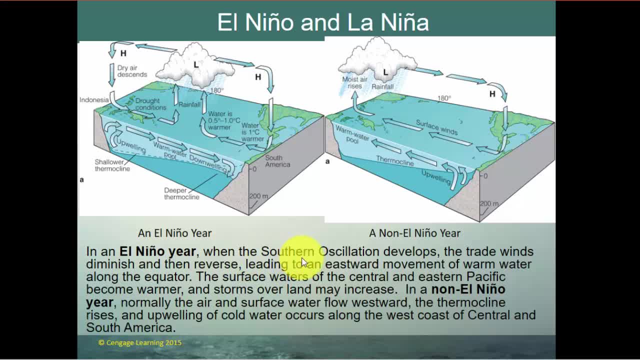 So let's read through this. In an El Niño year, when the southern oscillation develops, the trade winds diminish and then reverse. So what happens is the trade winds that are blowing in here. they weaken and reverse, And that allows all this warm water instead of flowing to the west. 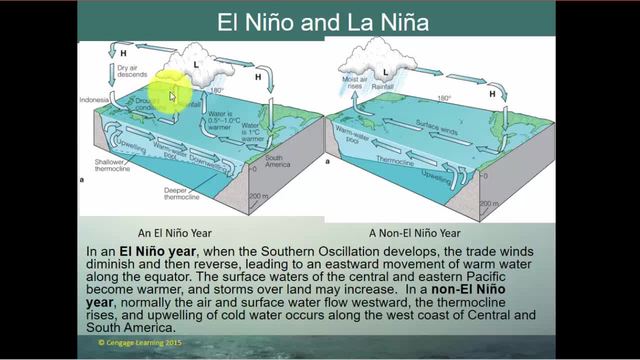 all that warm water flows back to the east And where all the warm water in a non-El Niño year is piled up on the west side of the Pacific with cold water over here in an El Niño year because the trade winds flip or reverse. 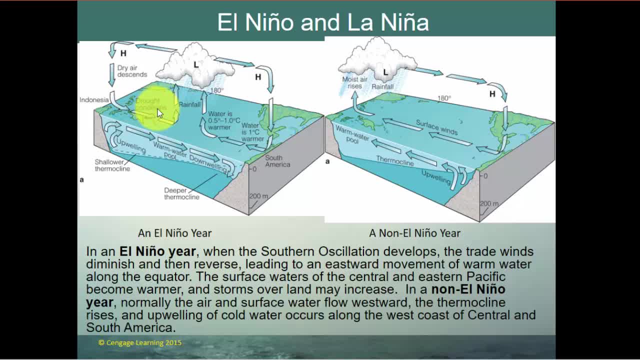 that's the oscillation. the winds blow back down that gradient and you get much, much warmer water over the central equatorial Pacific Ocean. In an El Niño year, when the southern oscillation develops, the trade winds diminish and then reverse. 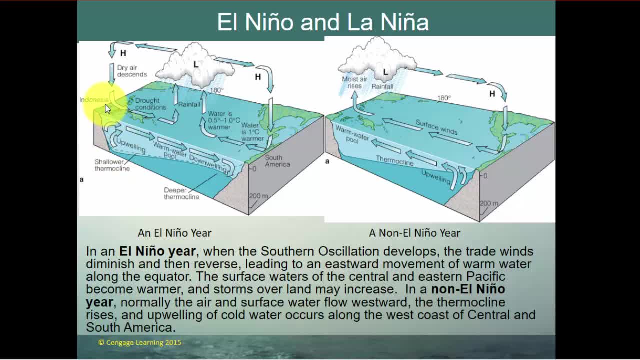 leading to an eastward movement of warm water along the equator. That is, the eastward movement, right there, of the warm water along the equator. The surface waters of the central and eastern Pacific therefore become warmer, and storms over land may actually increase. 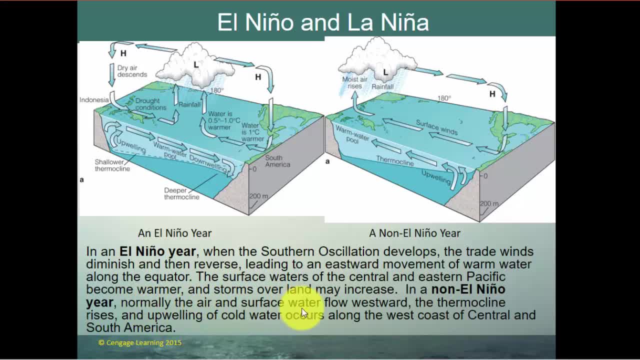 In a non-El Niño year, normally the air and surface water flow westward and an upwelling of cold water occurs along the west coasts of Central and South America. So this is the El Niño year, with this warm water flowing back toward the central and eastern Pacific. 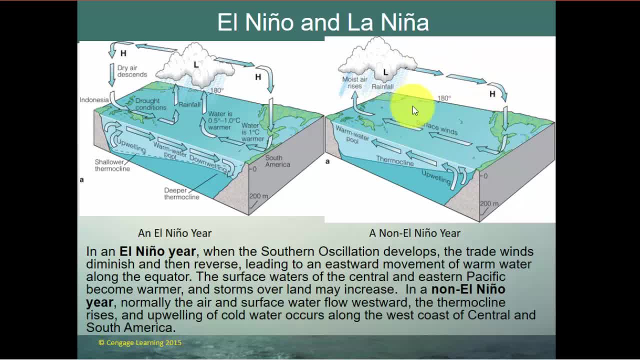 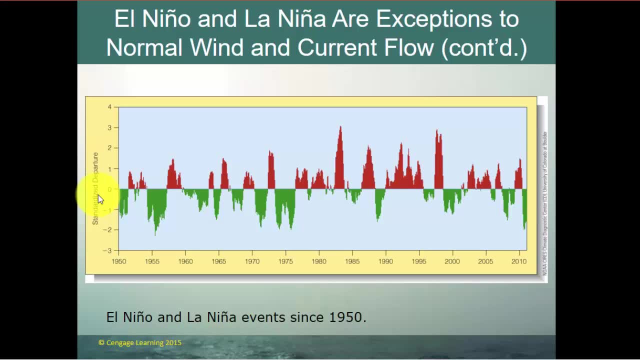 and in a non-El Niño year where all that warm water stays back here on the west side of the Pacific Basin. This is kind of the curiosity or how often those events happen. This goes back to about 1950 and we see the different El Niño years. 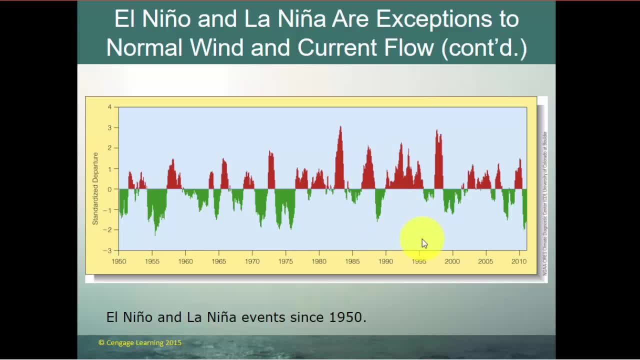 So in 1987 we had a big El Niño year and in 1998 we had a big El Niño year. So in 1987 we had a big El Niño year. So in 1987 we had a big El Niño year. 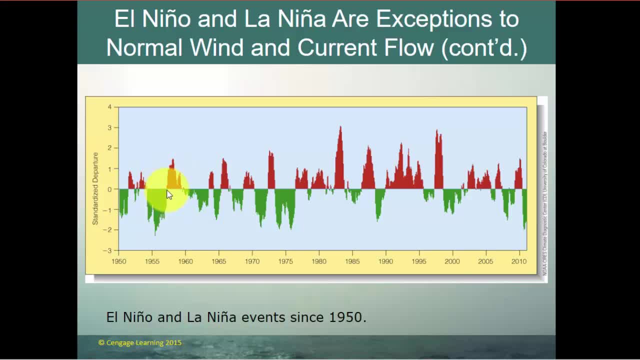 And you see that these El Niño periods may last for 3 or 4 to 7 years, and then the non-El Niño. So the equatorial Pacific goes from being warmer than normal to colder than normal, and warmer than normal to colder than normal. 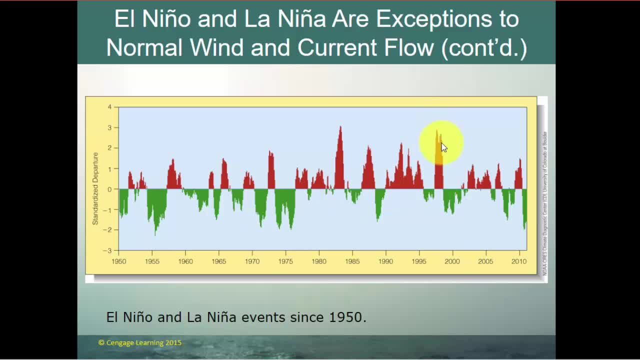 Here again: 1998, much warmer than normal, and then, through 2000, colder than normal, And then we had a period of warmer than colder, And so that is sort of the period of El Niño and non-El Niño years. 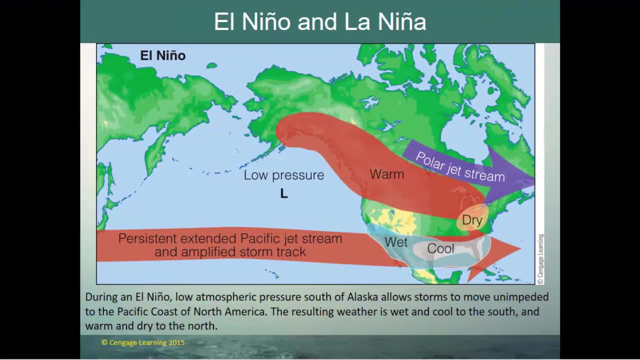 The impact of an El Niño season is the warming of the equatorial waters of the Pacific Ocean, So the region actually south of Hawaii, And that warming of that equatorial water creates a much stronger, persistent jet stream moving across this part of the Pacific Ocean. 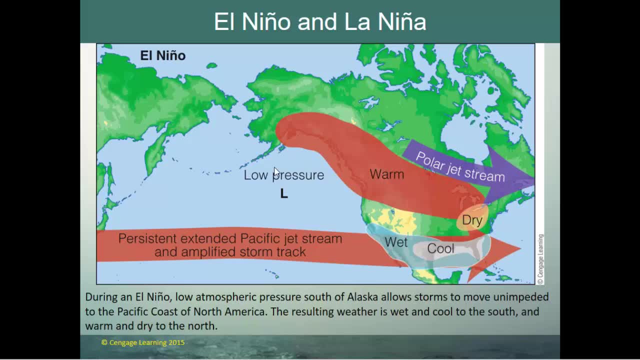 And with the low pressure that sets up south of Alaska, it just produces a very, very wet and stormy pattern that moves across essentially the southern tier of the United States. This strong wind also moves all the way across the Gulf of Mexico and into the Atlantic Ocean. 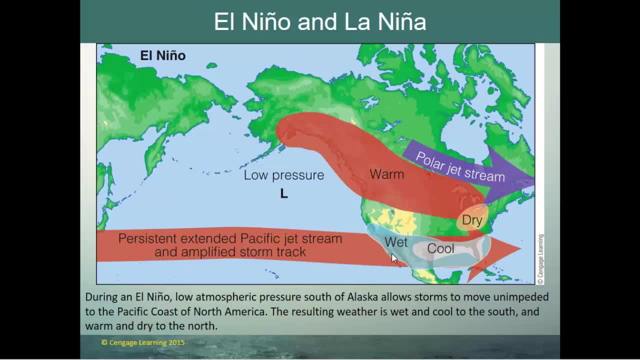 And during an El Niño year, this strong subtropical jet actually helps to reduce the number of hurricanes that form, or, if hurricanes do form, it tends to deflect them out into the Atlantic Ocean quickly, That is, in the Atlantic Basin. Alright, when we're talking about 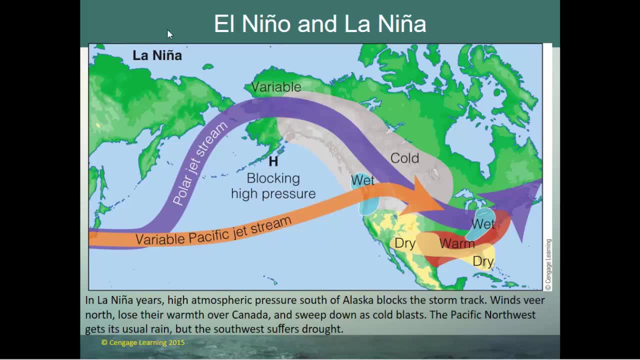 non-El Niño years- that La Niña I mentioned, but non-El Niño years. your more typical pattern is a large blocking high pressure area south of Alaska that causes the main storm tract to be deflected way to the north. 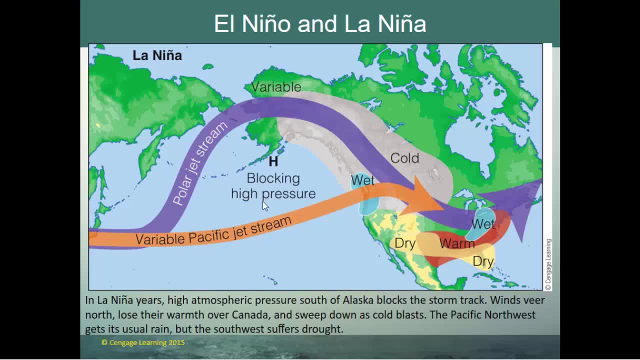 That keeps it much drier across the southern states and even warmer for us across the southeastern states, And this jet stream is much more variable, So oftentimes it comes in way to the north, So that subtropical jet A does not bring strong showers and storms. 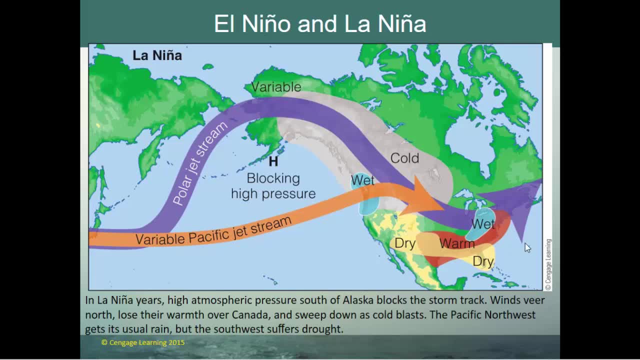 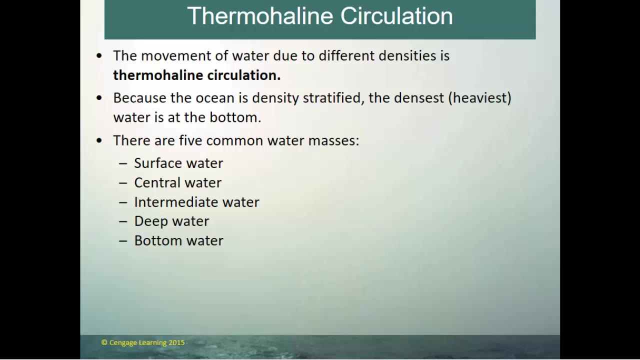 into the southern tier, but it also doesn't deflect or thwart the development of tropical systems in the Atlantic Ocean. So La Niña or non-El Niño years, we typically have a more active Atlantic hurricane season. Alright, so we talked a little bit about. 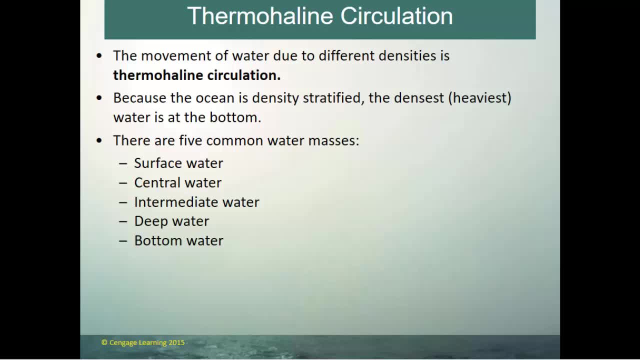 the vertical motion of water in the Atlantic due to wind. We talked a lot about the horizontal motion of water due to wind, the gyres and the ocean currents. Let's talk about how density differences cause water to move And those density differences create what's called the thermohaline circulation. 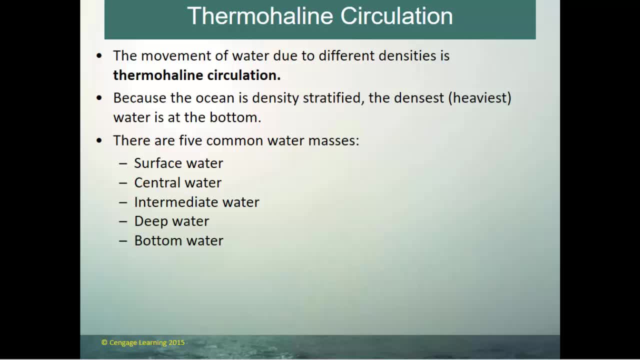 So, thermo being temperature, haline being salt, And what it means is the difference in temperature of the ocean water or the difference in salinity of the ocean water causes different density characteristics of layers of water, which causes the ocean to become density stratified. 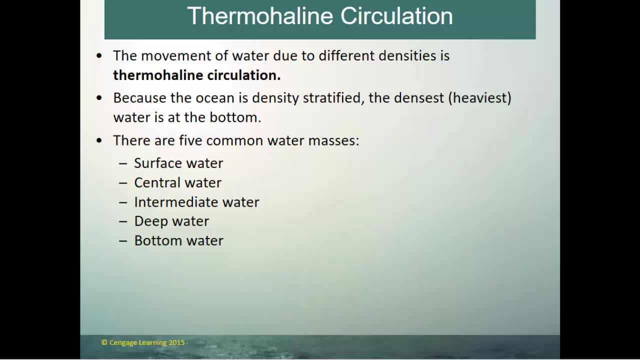 Meaning the densest water will be at the bottom and the least dense water will be at the top. So, because of these density differences, there are five basic water masses. You have your surface water, central, intermediate, deep water and then your bottom water. 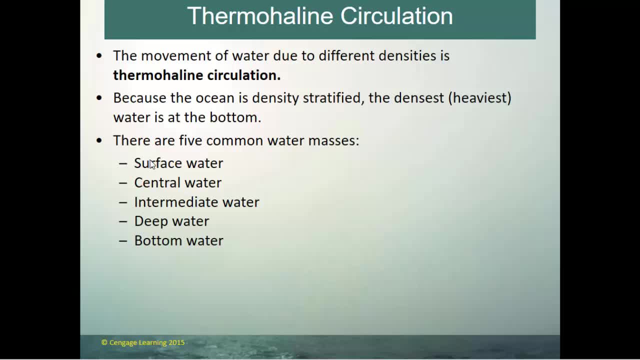 And, of course, the densest is going to be the bottom water and the least dense is going to be the surface water. The coldest and saltiest, the bottom water and the clearest, the least salty and the warmest, the surface water. 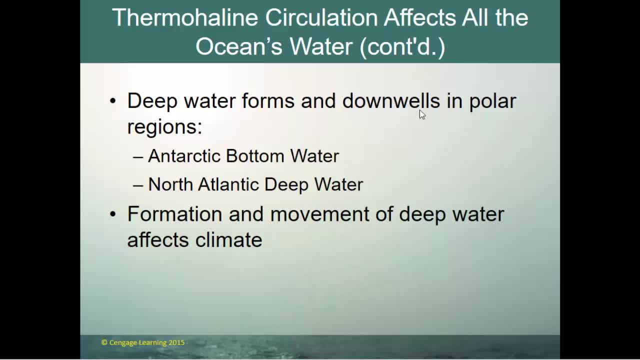 So deep water forms and then down wells in polar regions, Meaning when water gets up to the polar areas, it gets very, very cold and begins to turn to ice Well. when ice forms, only the pure water transition has a phase change from liquid to solid. 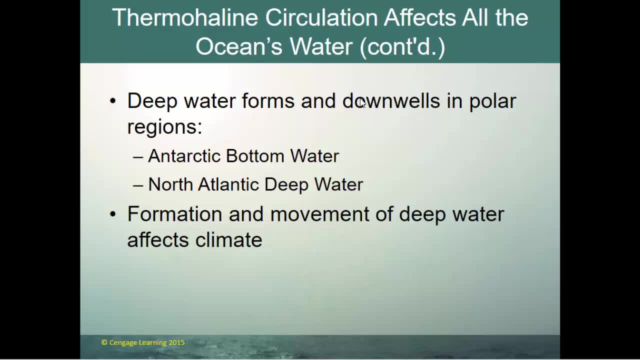 So of all the water in the polar regions that may have salts in it. as that water turns to ice, the salt is left behind, which means the ice forms, leaving behind very cold, very salty water that tends to down well or sink. So deep water forms and down wells in the polar regions. 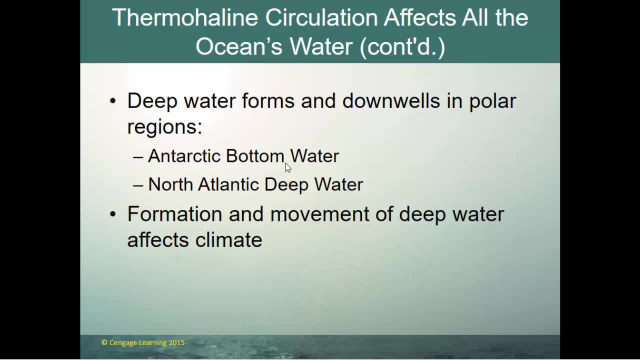 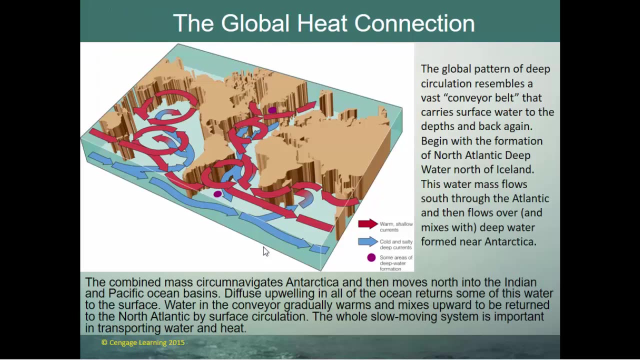 It becomes Antarctic bottom water or North Atlantic deep water, And this formation and movement of deep water definitely affects the climate. Alright, so this global circulation creates a global heat connection. So let's go through this. This is what's known as the great global conveyor belt. 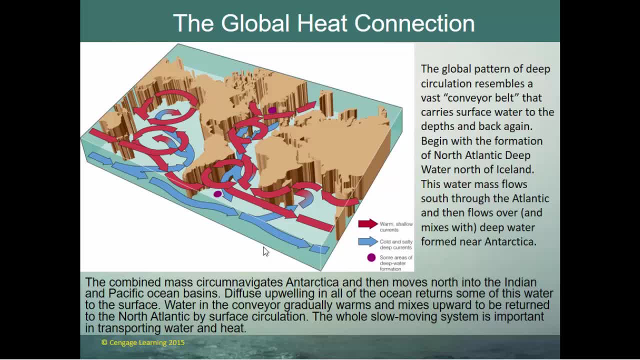 Essentially, the global pattern of deep circulation resembles a vast conveyor belt. That conveyor belt carries surface water to the deep depths and it does so in the polar regions and then back up to the surface again in the equatorial regions, So beginning with the formation of that North Atlantic deep water. 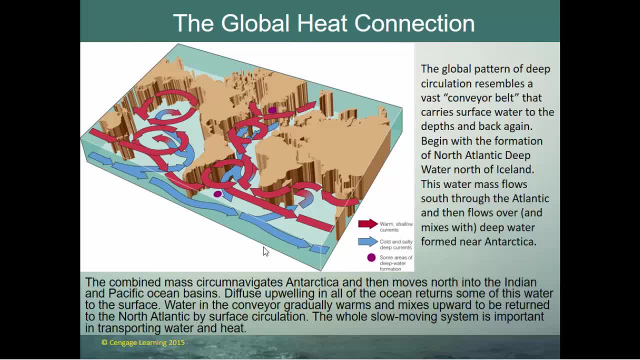 so that's that water in the North Atlantic that freezes becomes very salty. what's left over becomes very salty, cold and dense and sinks Forms that North Atlantic deep water, And that's going to happen again up in the North Atlantic. So that's the water that comes up. 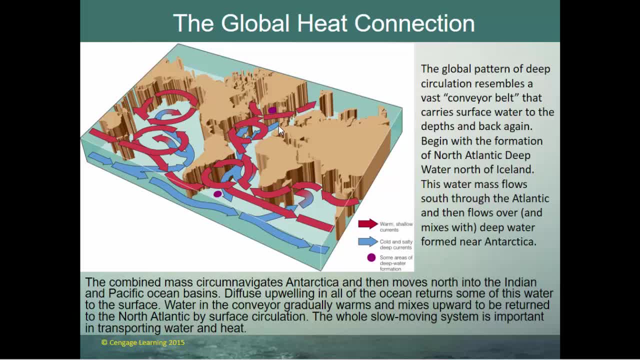 it freezes and it sinks, creating this blue arrow here, the North Atlantic deep water, which then flows south under the force of gravity Water north of Iceland, that's what we're talking about. This water mass then flows south along the Atlantic and then flows over and mixes with the deep water. 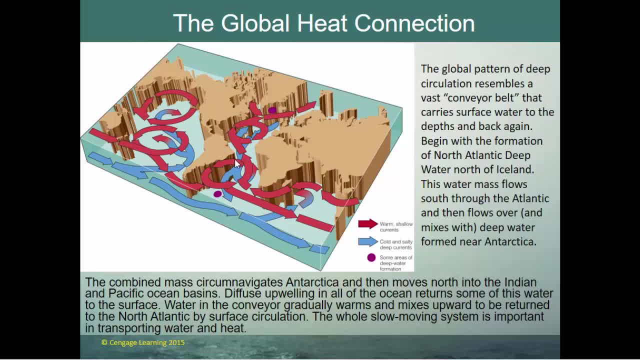 formed near Antarctica. So it flows south and mixes with this deep water near Antarctica. The combined mass- that's the two, the North Atlantic deep water and the Antarctic deep water bottom water- the combined mass then circumnavigates, goes all the way around Antarctica. 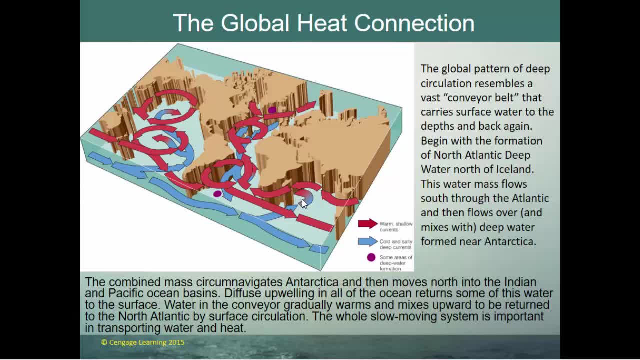 and then begins to move north into the Indian Ocean and also in the Pacific basins. Water gradually warms here and mixes upward to be returned to the North Atlantic by surface circulation. So it mixes upward and the Atlantic flows around that gyre, gets caught up in the southern gyre. 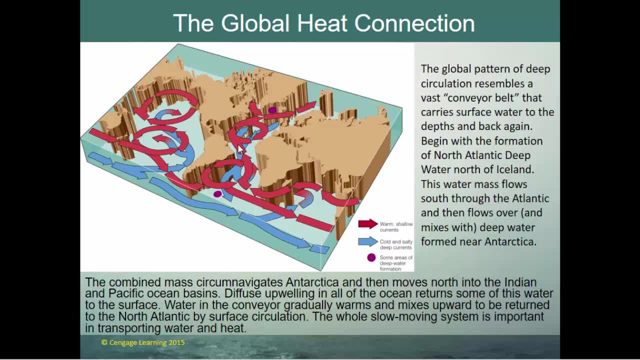 maybe flows around South America into the South Atlantic and eventually up into the North Atlantic. So you start out very cold. you drop to the bottom, you mix with the Antarctic water, you move up in the Indian Ocean, you move over into the Pacific Ocean. 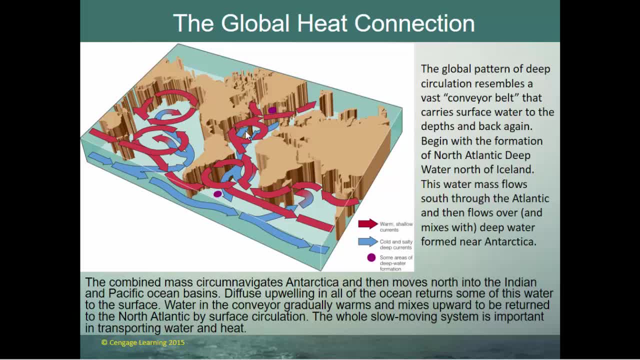 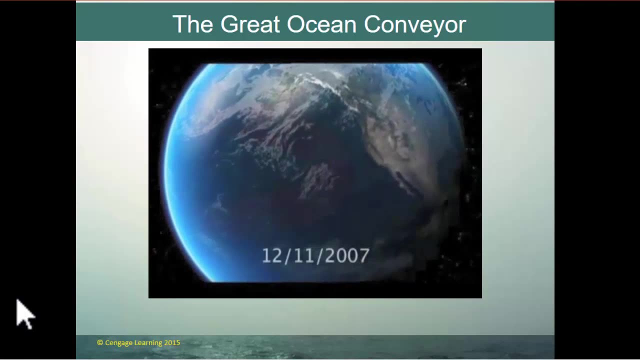 you rise back to the surface as you warm and eventually you connect back up into the North Atlantic where the whole process starts over again And the whole very slow moving system very important for moving heat north and cold back to the south. It's called the Great Ocean Conveyor. 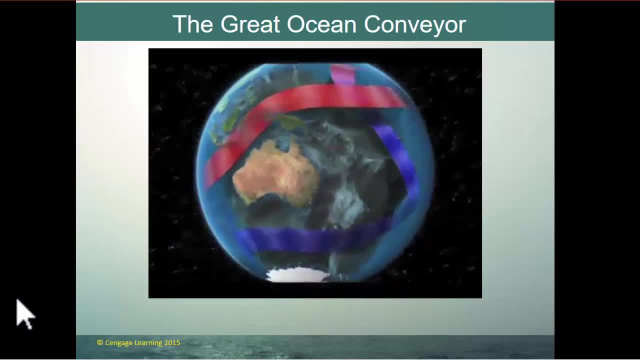 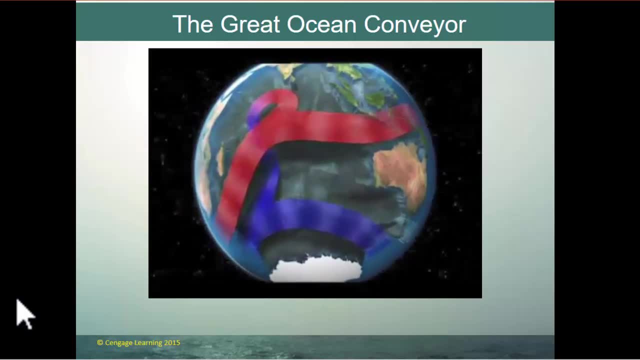 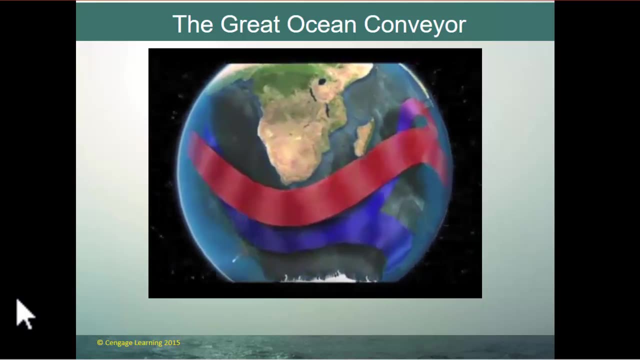 and it's one of the most powerful forces on the planet. It's made up of warm currents which travel at the surface, whilst at the bottom of the ocean are much colder currents. The conveyor transports oxygen, nutrients and warmth around the world. It's vital to the health of all life on Earth. 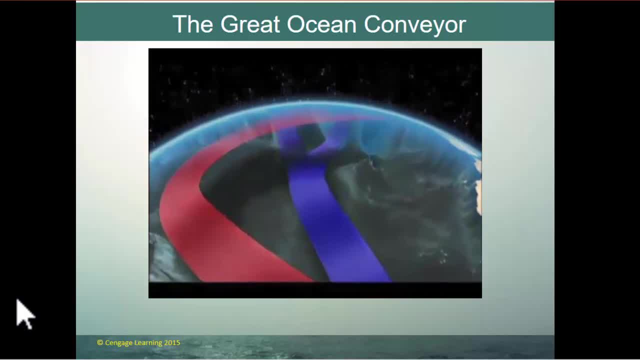 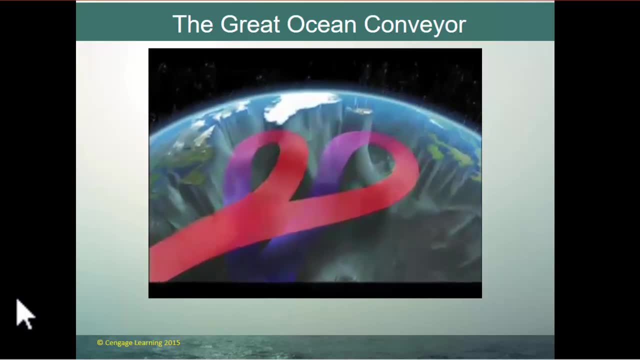 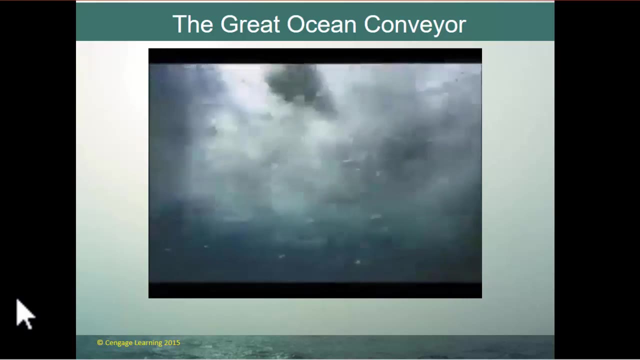 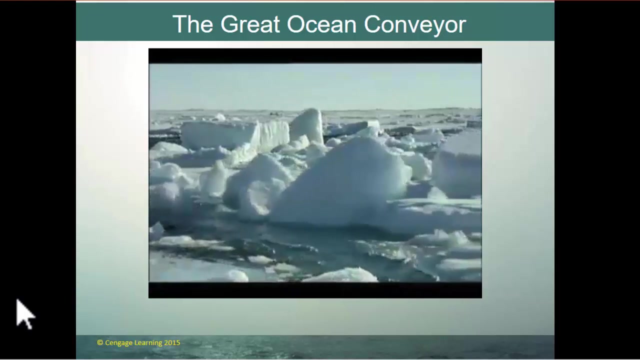 Yet the conveyor wouldn't keep flowing if it wasn't for what happens in the cold northern oceans. This is where the surface water sinks to join the deep water currents. The sinking happens because the water's very cold. This makes it dense and heavy. 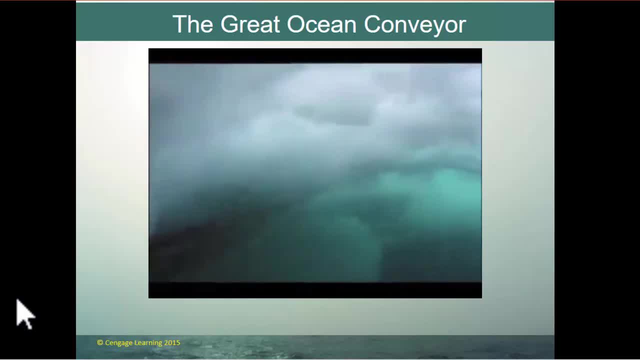 so it plunges to the bottom of the ocean, And it's this sinking water which keeps the entire conveyor moving. As it travels south, it hugs the ocean floor until it warms at the equator, where it eventually rises to complete the circuit. 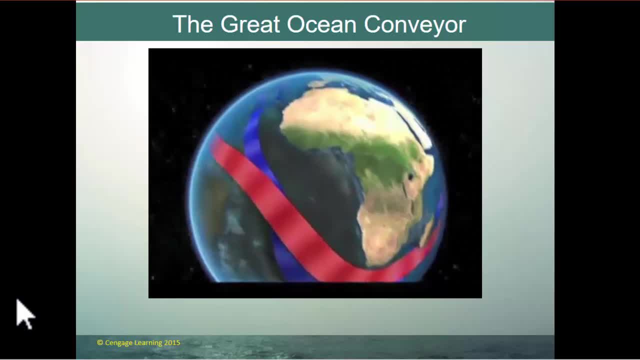 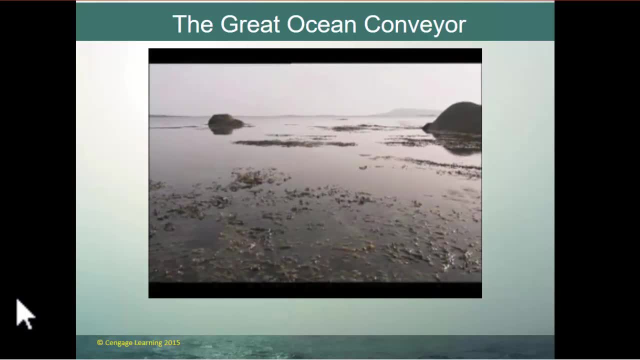 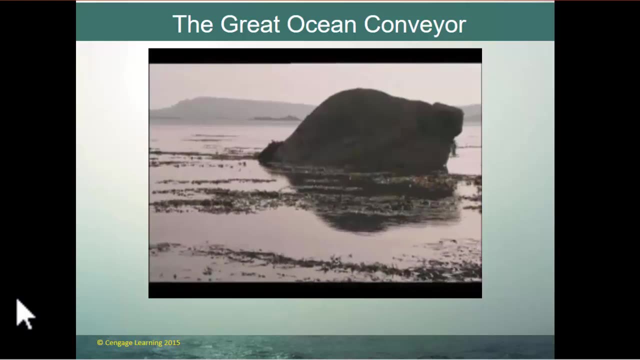 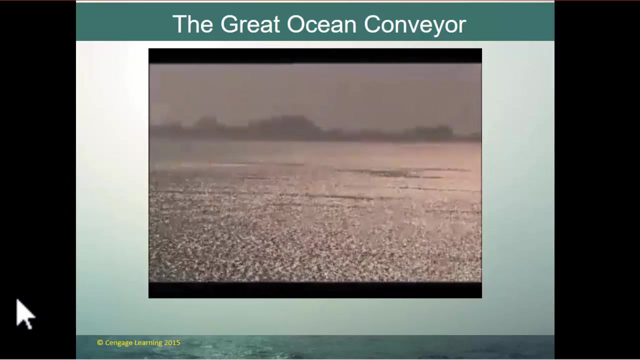 Without cold water sinking at the poles, the ocean conveyor would collapse. The sea would no longer be supplied with oxygen and nutrients. It would become stagnant and lifeless. It takes roughly a thousand years for water to circulate all the way around the conveyor. 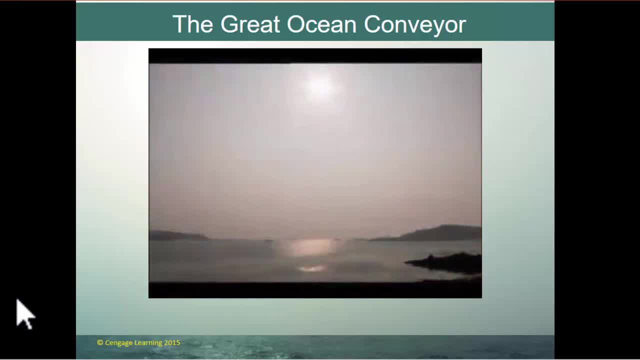 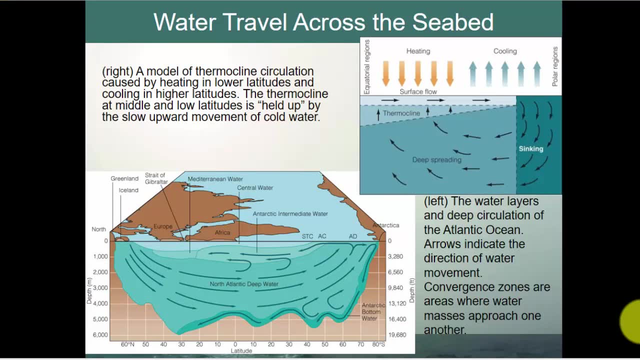 And this global network of currents controls the well-being of the entire planet. Without it, our world simply wouldn't function. So a couple different illustrations of how the water travels, not only across the surface, but also over the seabed. At the left, the water layers. 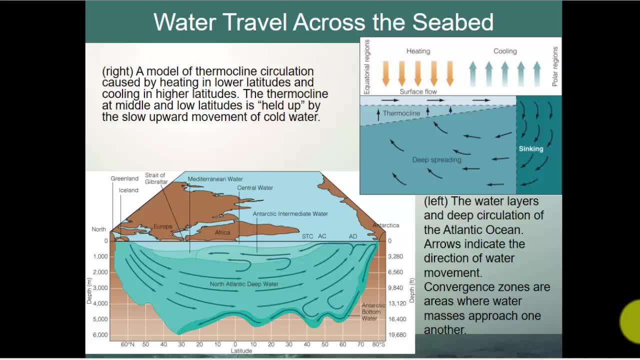 in deep circulation of the Atlantic Ocean here. So we see where water sinks in the northern parts of the Atlantic Ocean, up near Greenland and Iceland, as salty water turns to ice, leaving behind very salty, very cold water which is more dense, and so it sinks. 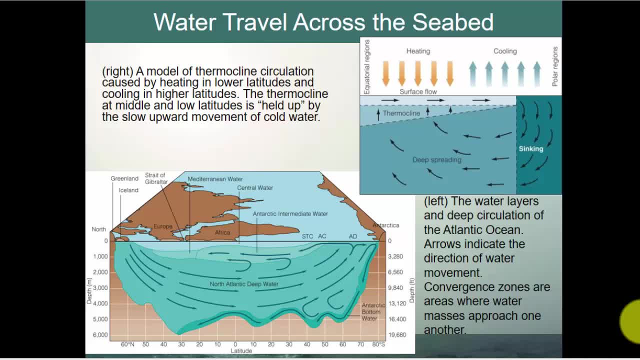 It sinks down at the bottom of the Atlantic Ocean and then flows south until it gets down to about Antarctica, where the same processes cause water to sink. in Antarctica, The water turns to ice, leaving behind cold, salty water. It sinks. Those two masses mix. 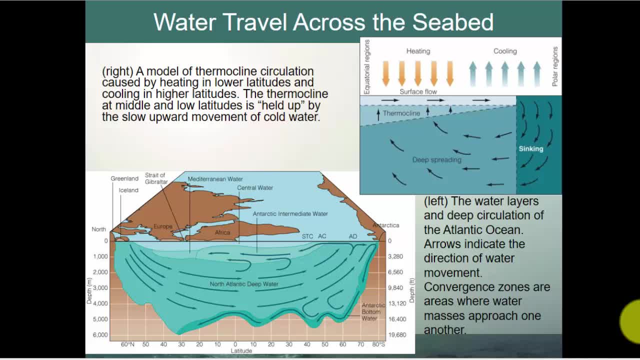 The Antarctic bottom water and the North Atlantic deep water. they mix, And then they travel either over into the Indian Ocean or the Pacific Ocean, and then some upwelling and warming brings them back up to the surface, creating the entire circulation. And so, to the right, you have a model. 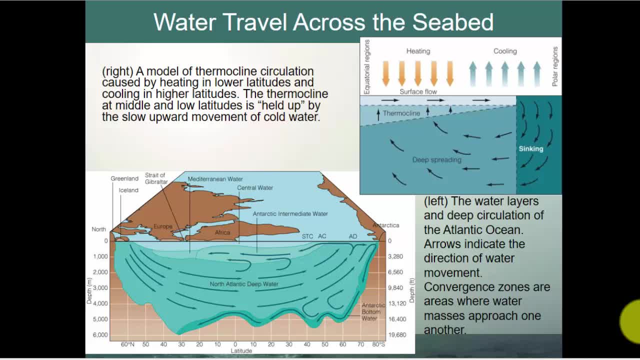 of the thermocline circulation caused by heating in the low latitudes. So here you heat the water up, it becomes less dense, and then chilling in the higher latitudes that causes the water to sink And again. so these differences in both salinity. 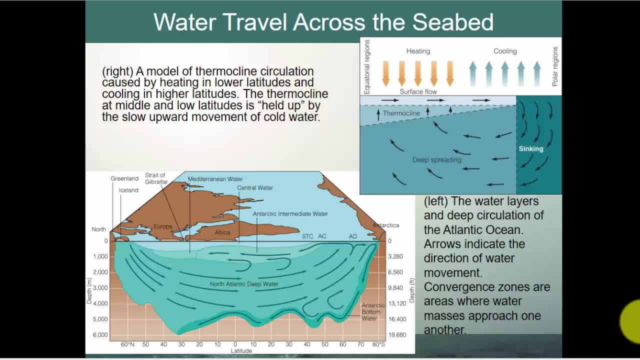 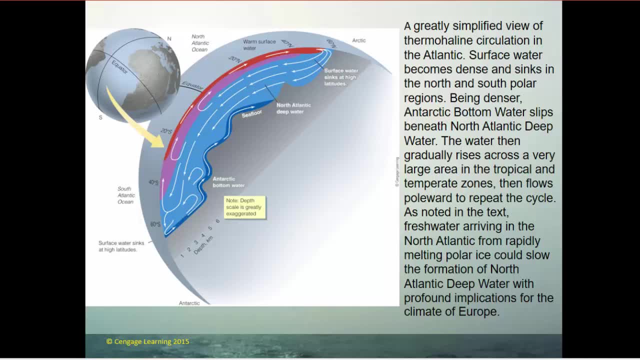 and in temperature create density differences that cause this water to move around the globe, the global conveyor belt- And here's a very simplified view of the thermohaline- both heat and salt, or heat and salinity, temperature and salinity circulation in the Atlantic. 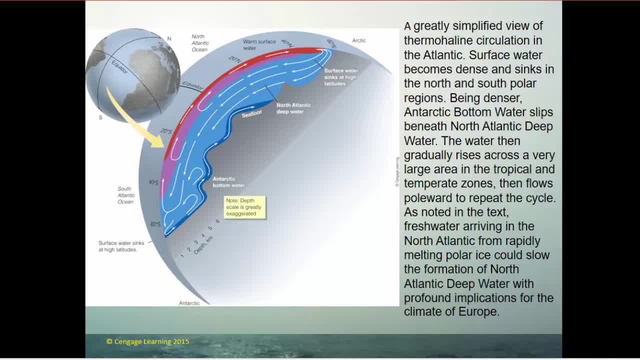 Surface water becomes dense and sinks at the north and south polar regions. being denser, Antarctic bottom water slips beneath North Atlantic deep water and the two kind of mix to some degree there. The water then gradually rises across a very large area in the tropical temperate zones. 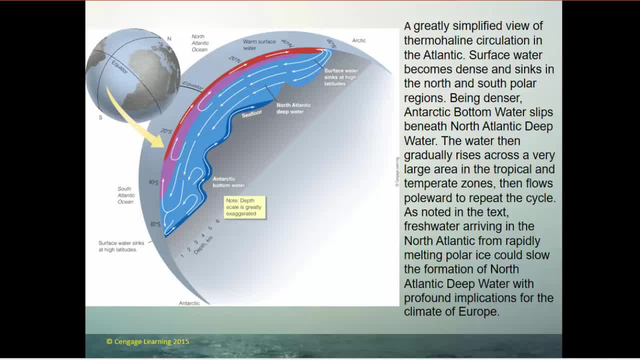 then flows poleward to repeat the cycle. As it talked about in the text. fresh water arriving in the North Atlantic from rapidly melting polar ice could slow the formation of the North Atlantic deep water, with big implications in the climate of Europe. So what that's telling us is: 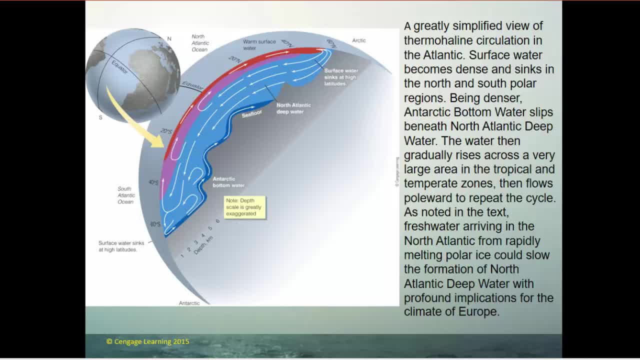 that if the climate warms to a degree that the polar regions see a great deal of ice melt, then all that fresh water that would come from that ice melt would then cause that North Atlantic deep water to form more slowly, because there wouldn't be the density differences. 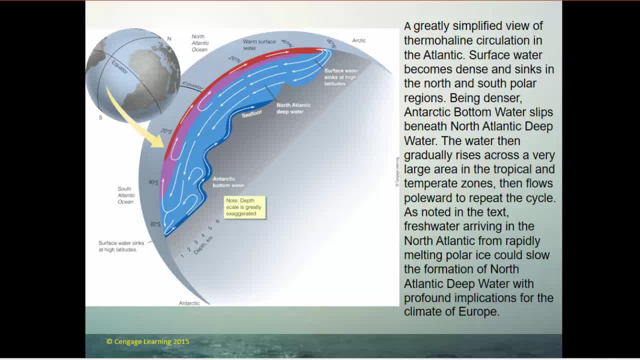 and that could cause some big impacts in terms of chilling the climates of Europe. So that's one of those interesting feedback mechanisms where the warming of the globe may cause the melting of polar ice, but the melting of polar ice actually slowing down the global conveyor belt. 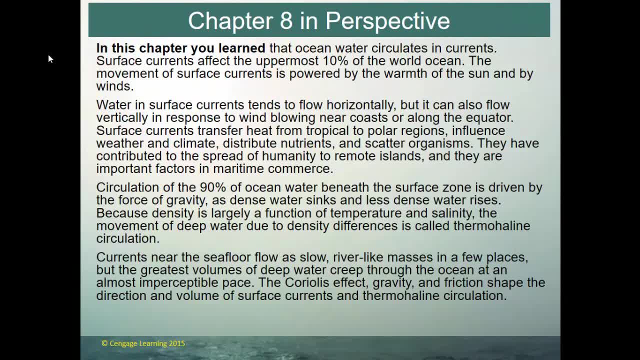 and therefore cooling Western Europe. In Chapter 8, we've learned that ocean water circulates in currents and that surface currents affect only the uppermost 10% of the world's ocean. The movement of surface currents is powered, ultimately, by the warmth of the sun. 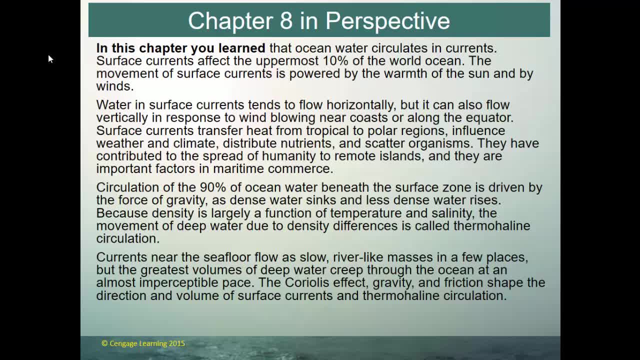 but it's the warmth of the sun and the differential heating of the Earth's surface that causes the winds, and the winds are what effectively cause the ocean currents to begin moving. Water in surface currents tends to flow horizontally, but we also learned that horizontal movement of water